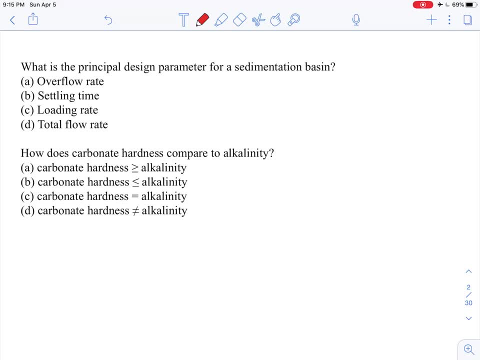 So maybe a lot of you, when you saw the sedimentation, you think of the particle settling right because of the gravity. So you may choose the settling time of the as a principal parameter. But if we talk about the design parameter then you can see from the textbook and also from my notes that for the sedimentation basin we're mainly using the overflow rate. 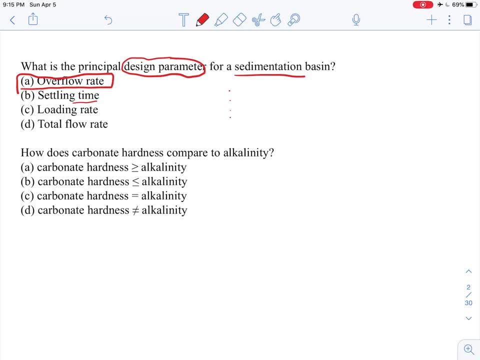 Or the surface overflow rate as the principal design parameter for the sedimentation basin. So this should be, so A should be the answer of this problem. So the second question is asking: what is the relationship between carbon and hydrogen? So the first one is the carbon hardness and also the alkalinity. 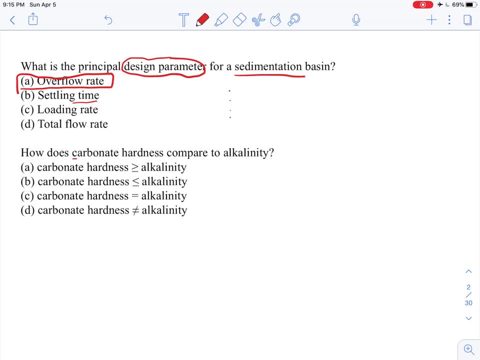 So if you, basically, if you look at the definition of the carbonate hardness, So it's defined as the parameter or the is defined as the total, either total hardness or alkalinity, whichever is smaller Right. So the carbonate hardness Right Is total hardness. 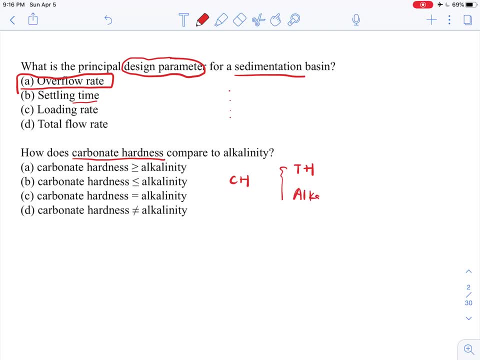 Or alkalinity. So basically the minimum Of these two right, whichever is smaller. So this means that if alkalinity is above the total hardness, then the carbonate hardness is equal to total hardness, which means that the carbonate hardness is smaller than alkalinity. 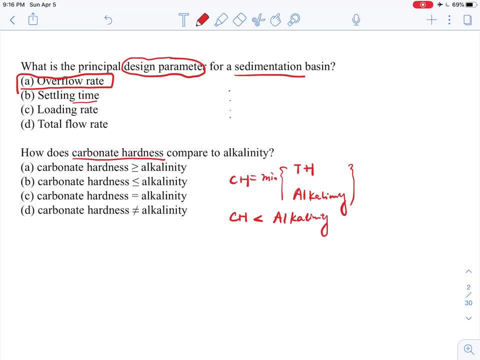 And if the total hardness is higher than the alkalinity, Then the carbonate hardness is equal to the smaller one. So under that situation the carbonate hardness is equal to alkalinity. So after combining these two we can see that actually B is the correct answer. 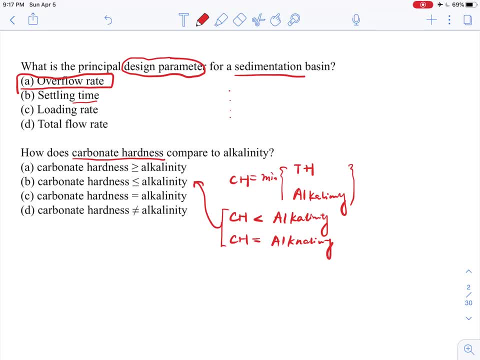 You may say that there's a lot of definitions here, Right? So it is not a direct way of showing what is the relationship here. So let's give two examples here. OK, so we talk about the hardness. Hardness are mainly just the calcium and magnesium in water. 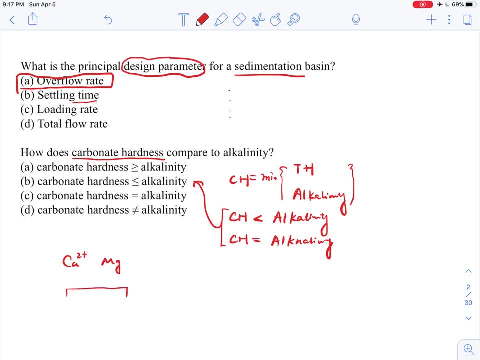 Right, So we create that bar graph that's showing the relationship between the cations and anions, Right? So let's say this is a cations, Right? So if we have a situation where the carbonate hardness Is here, So the rest of it are going to be some other types of anions. 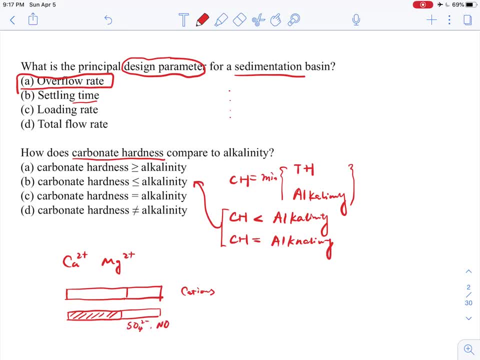 Right. There can be sulfate, Right, Nitrate, So on and so forth, And here is bicarbonate, Right. So under this situation, the carbonate hardness is equal to the alkalinity Right, Because in this water, here, since we have these two ions, 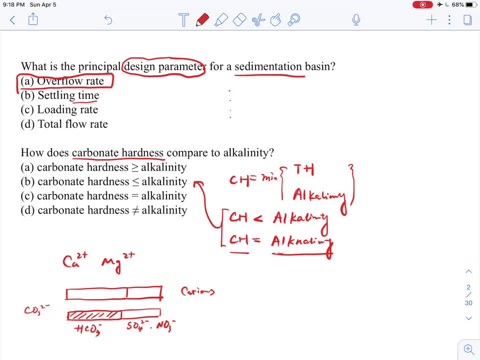 there are no carbonate ions here And there's, we can assume that the pH is close to seven, which means that the OH ion concentration is much smaller than one which is negligible. OK, So under this situation, the carbonate hardness is just equal to the alkalinity. 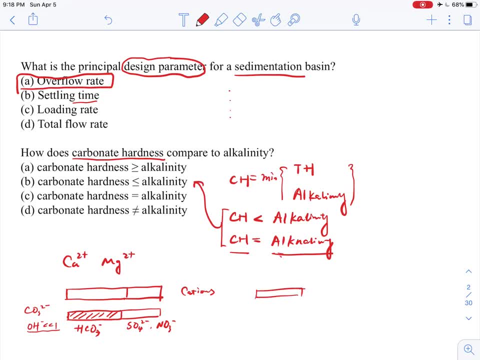 So we can also have the situation where, Let's say, this is the calcium, Magnesium Right, And we have carbonate or bicarbonate ions that has a much higher concentration. So what this means is that the remaining cations can be sodium, potassium or so on. 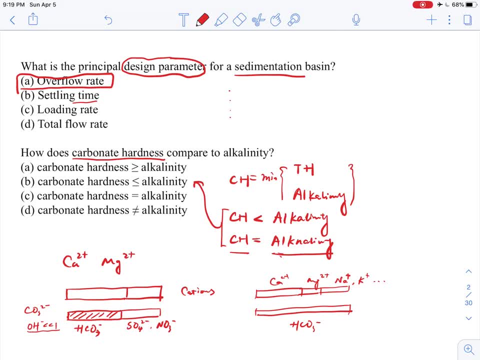 But if you think of the definition of the carbonate hardness. So basically these types of ions, they're not going to contribute to the hardness of water Because they're not forming sedimentations. when we boil the water Right, When you heat it up, you're not seeing these sedimentations. 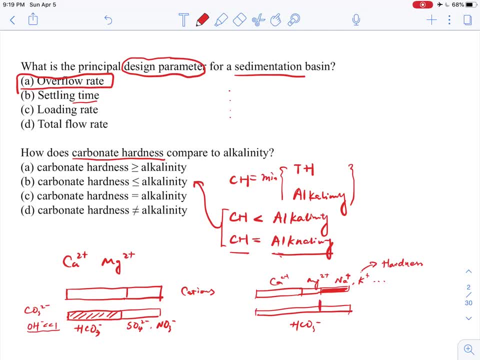 So what that means is that the carbonate hardness is just here. OK, So under this situation, the carbonate hardness is equal to the total hardness, And by showing that, we can see that the basically, in this way, the carbonate hardness is smaller than the alkalinity. 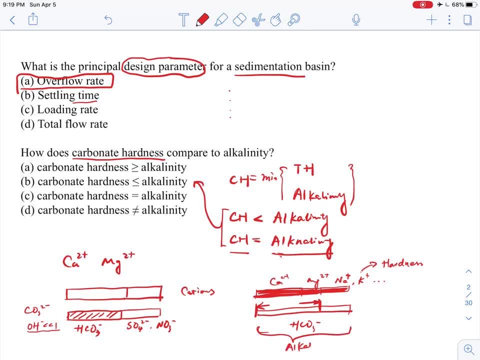 Where the alkalinity is here Right. So this is giving us the correct answer, which is B here. So these two are the two major problems that I saw. So there's another problem about evaluating the river water quality. So people will typically prefer late summer to do those measurements, because the water level is the lowest. 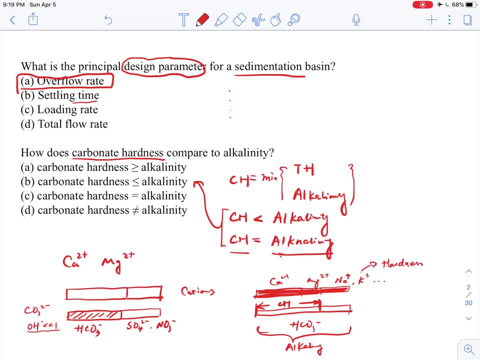 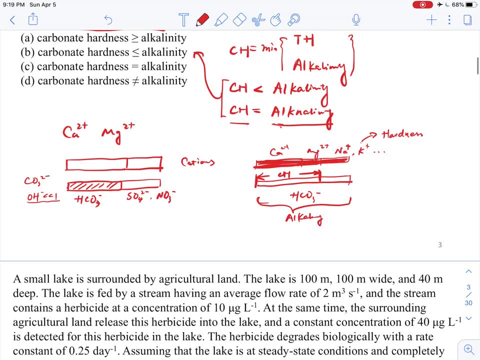 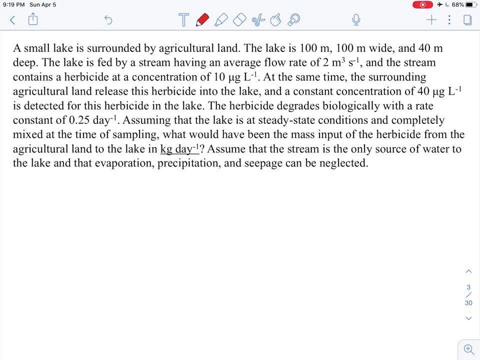 And also the reaction rate are the highest. So there's a bunch of reasons why people Would like to do the water quality evaluation at late summer. OK, And in terms of the calculation problems, I think a lot of you must have watched my review session that I posted last week. 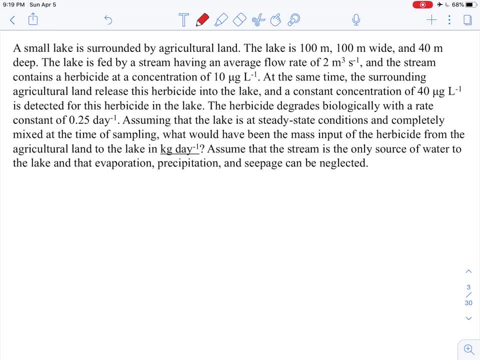 So I'm glad to see that you are following those steps. But there are some differences in these calculations here. So for example, for the first problem a major difference. So apart from these geometry here, I remember that for the other problem, 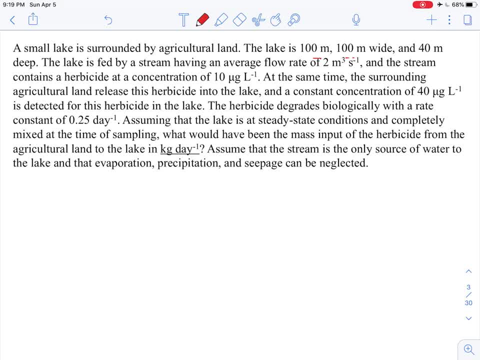 the depth is 30, right, And the lands and waves are also different here, Also in terms of flow rate, But the major difference is this inflow concentration here. So if we read again from the beginning on this problem, So let's say that there is a small lake. 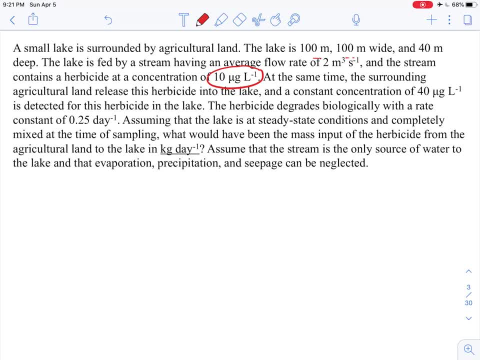 It's surrounded by agricultural land, So the lake is a square shape. Right It has a square shape in terms of the surface And also it has certain depths. Right We have 100 meters on the sides Right And 40 meters as a depth. 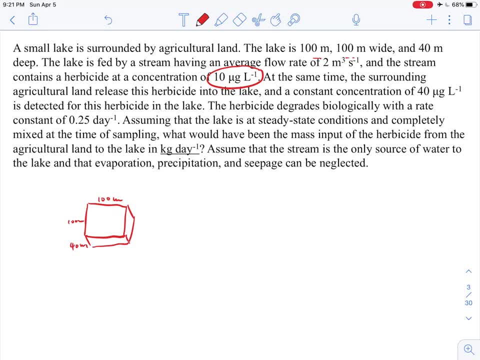 OK, So the lake is fed by a stream that's having an average flow rate of 2 cubic meters per second. So let's say this is the inflow, which is 2 cubic meters per second. Right? So because of the mass balance, 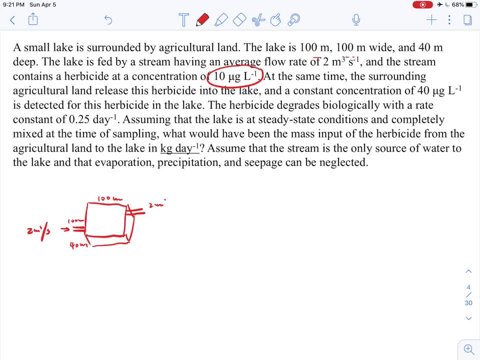 there must be an outflow which is also 2 cubic meters per second. OK, So I think almost all of you know this mass balance situation here. So it also says that the stream contains. so basically, this inflow stream contains a herbicide as a concentration of 10 micrograms per liter. 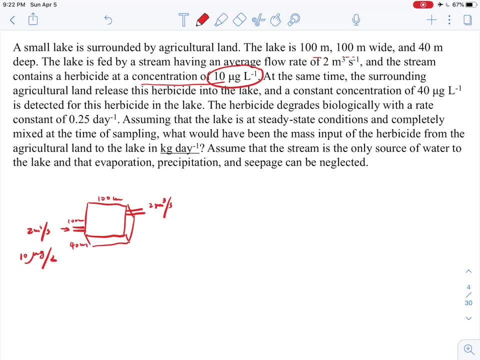 OK, Let's list it here Right. And also, at the same time, the surrounding agricultural land is releasing the herbicide into the lake And people are observing a constant concentration of 40 micrograms per liter in this lake. OK, So also we know that the herbicide degrees biologically with a rate constant of 0.25 per day. 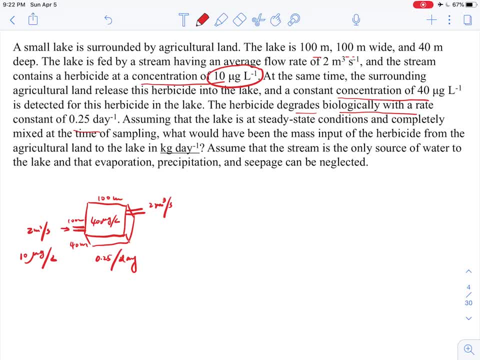 So we mentioned in our review session that, based on this unit here, we know that this is a first order reaction. OK, So, assuming that the lake is a steady state condition, what would have been the mass input, Right? So the mass input is asking about what is the total amount of herbicide that the agricultural land is inputting into this lake here? 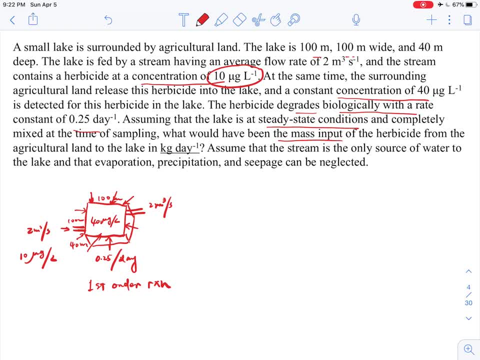 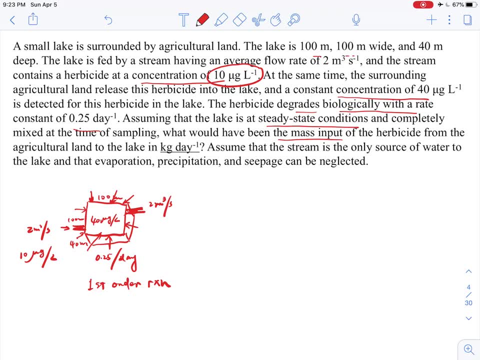 So we need to do a mass balance. So first, based on the mass balance of the water, we know that whatever flows in has to flow out at the same flow rate here, Right, And we need to also build a mass balance for the herbicide here. 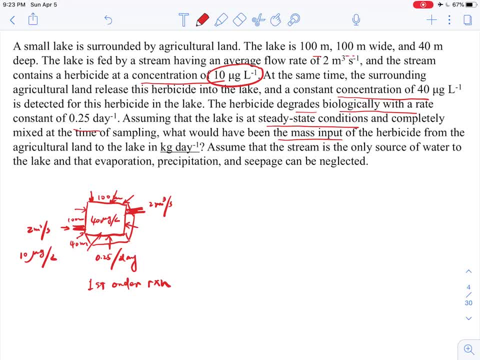 So let's say that we're trying to build up this equation. So basically, let's say the CH is the herbicide concentration, Right As a change, as a function of time. So we need to multiply that by the volume, which means that this is the total change of the. 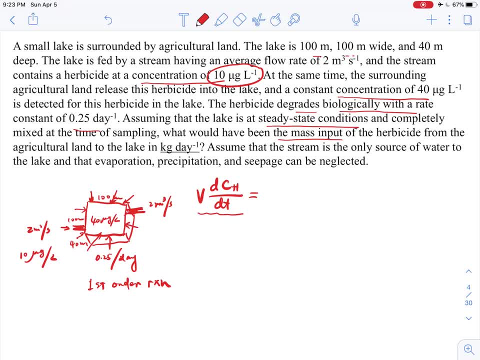 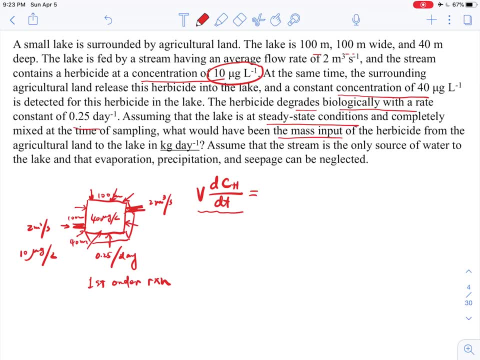 let's say the mass of the herbicide in this lake here. So this change is contributed. let's say this term is positive, then that's basically caused by the contribution, Right? So the contribution we can see that it's one part of it is the inflow. 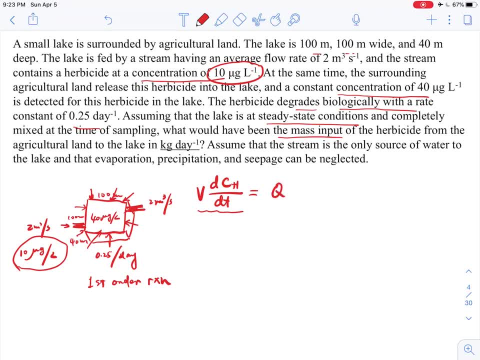 Right, We need to multiply. that is equal to Q multiplied by the concentration of the herbicide in that inflow. Okay, So it's asking for the mass input of the herbicide. So this is also the contribution of the herbicide into the lake. 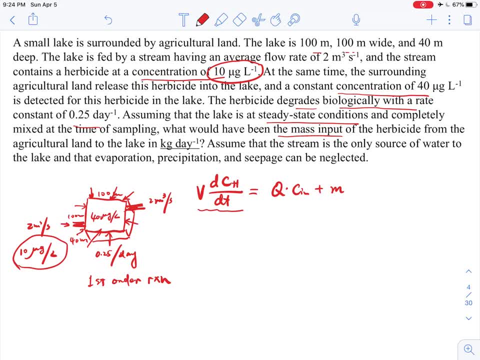 So there's also sinks. So basically these herbicide also are also consumed. So on one hand it's being consumed by this outflow, because the outflow is always pulling these herbicide outside Right. So we need to minus the Q multiplied by C out. 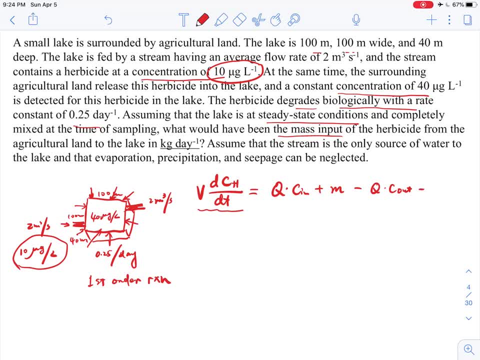 Right, And also we need to consider the reaction or the decay of this herbicide. We mentioned that this is a first order reaction, So we can calculate that by multiplying the volume of lake multiplied by the reaction rate constant and the concentration of the herbicide in the lake. 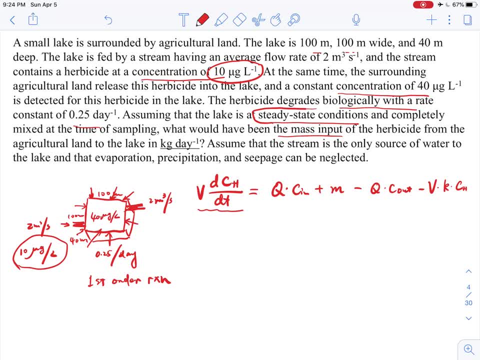 Okay, So further this problem, saying that the whole system is a steady state, which means that this is equal to zero. All right, So, which means that these four terms should be equal to zero. And since this is well mixed, it's also assuming that the herb in the lake is also well mixed. 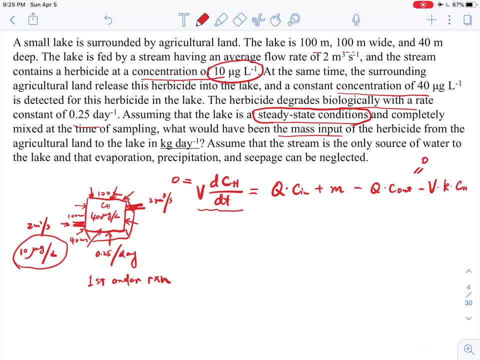 This means the concentration of the herbicide in the lake should be equal to the concentration of the herbicide in the outflow stream, Right? So we can further write out as: Q- C in plus M minus Q, C, H. Right, That is the concentration of herbicide in the lake minus V K, multiplied by C- H. 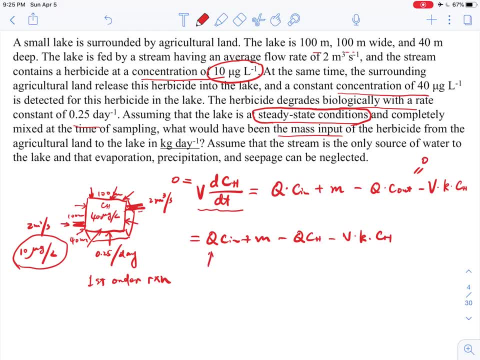 So now we can start to plug in all of these numbers. So we know that the Q is. We know that the Q is two meter cube per second Right. The concentration of the inflow is 10 microgram per liter Right. 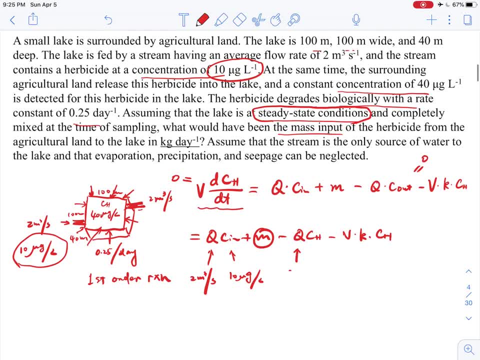 We're trying to solve for the M. So for the outflow, the flow rate is two meter cube per second. Right For this concentration. we know that this is constant Right- 40 milligram per liter Right. So for the volume, 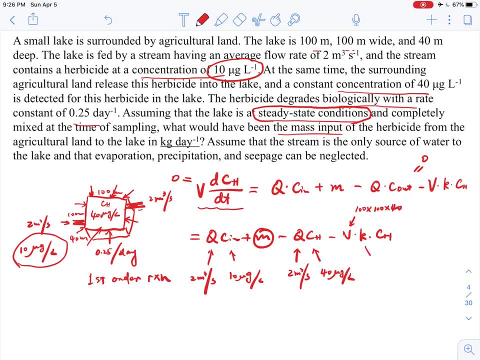 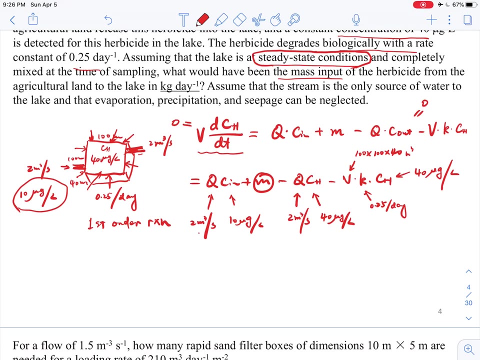 we can calculate that by 100, multiplied by 100, multiplied by 40. And then the K is 0.25 per day, Right? And then the concentration here is 40 milligram or microgram per liter. Okay, So we have to make sure that all of these units are under the standard units, because you cannot directly multiply these meter cube by liter here. 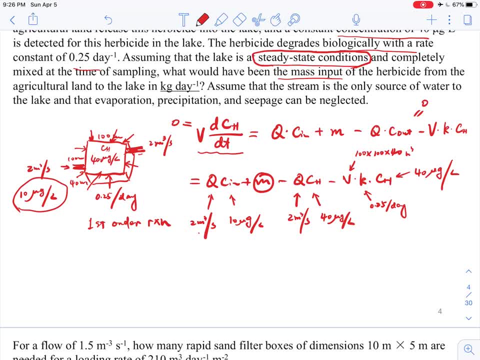 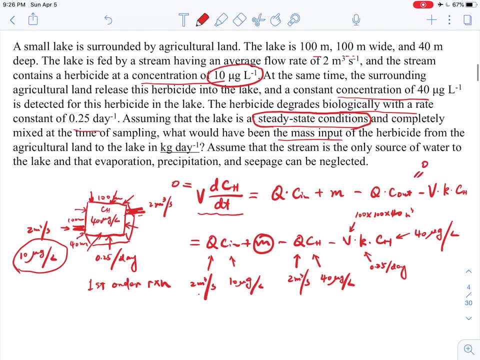 Right, You need to convert these, all of these units Under the same standards or the same set of units. So you can see that the major difference from the review problem that I posted in our review session is that for that problem we don't have this inflow here, because we assume that the inflow didn't have any herbicide concentrations there. 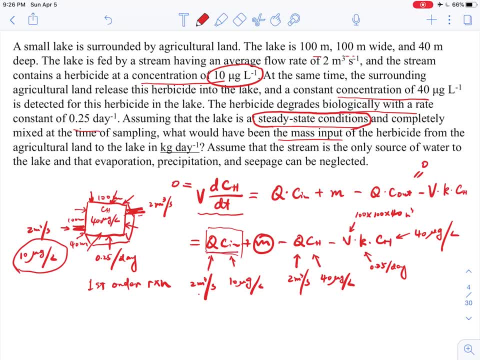 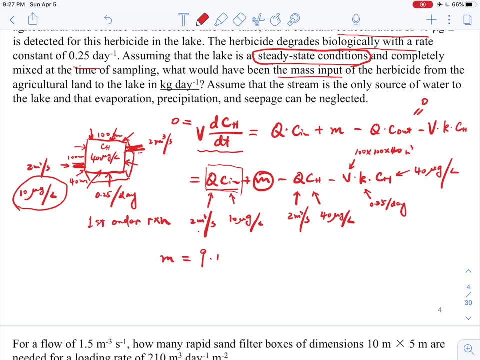 But for this problem there is a concentration Right, So because of that, the solution is different, which is going to give us a mass, A mass input of 9.18 kilogram per day. Okay, So this is the mass input of the herbicide from the agriculture land. 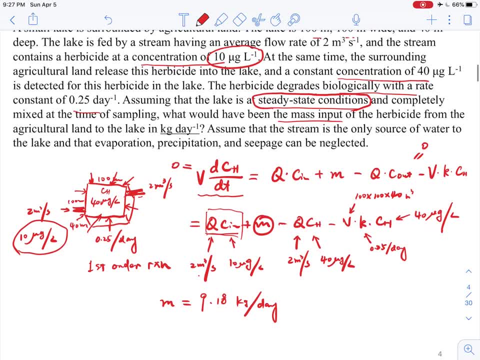 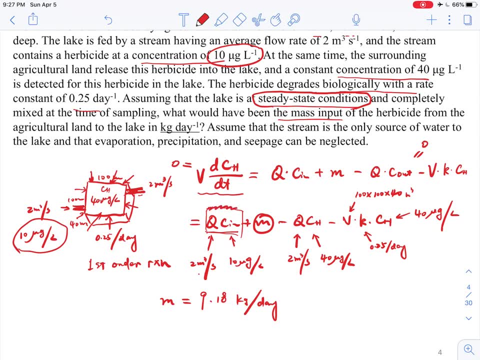 Right, So you can go through these calculation problem again just to confirm that this answer is correct. So I saw that a lot of you basically forgot about this term here And some of you assume that or treat this mass input as the rate change. 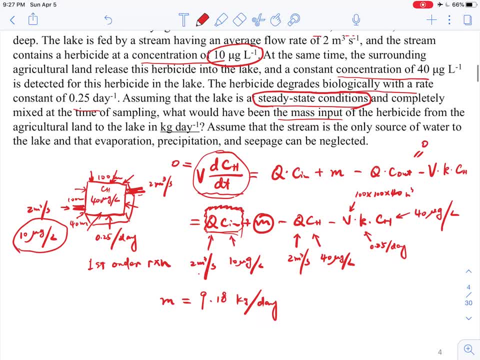 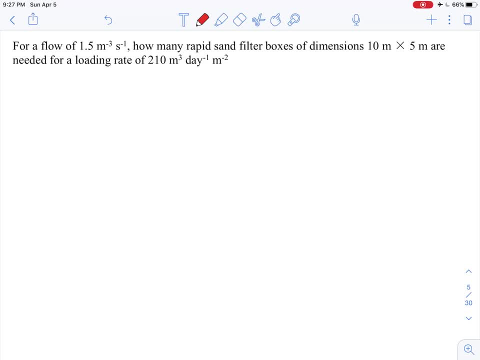 But that is not the case. Okay, So the other problem I want to talk about is basically this design problem for the represent filter boxes. So we had a similar problem for the homework practices. So the numbers here are a little bit different, but actually it's a little bit trickier when you're trying to solve for the answer here. 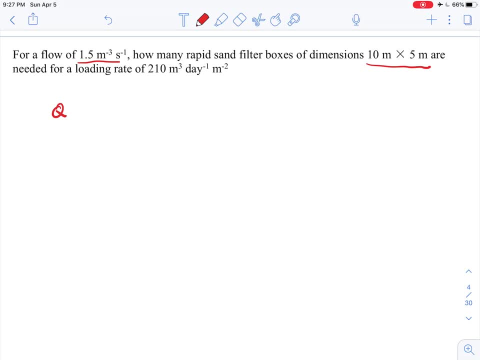 So basically, we have a total flow rate, Right. Total flow rate is 1.5 meter cube per second. Right, We have the loading rate. So the loading rate is, let's say the loading rate is 210 meter cube per day per meter square. 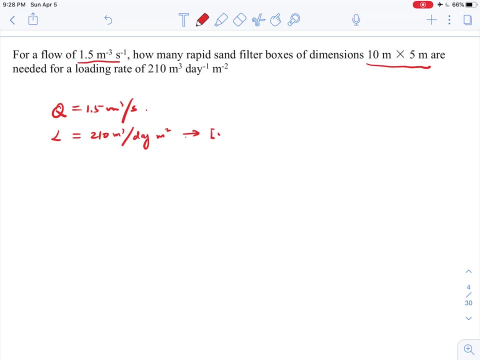 Okay. So basically this will give you a unit of meter per second, Okay, After you convert this day to seconds. So based on that, you can directly divide this Q by L to calculate this surface area. Okay, So you can calculate certain value here and further give you the dimension of this filter box. 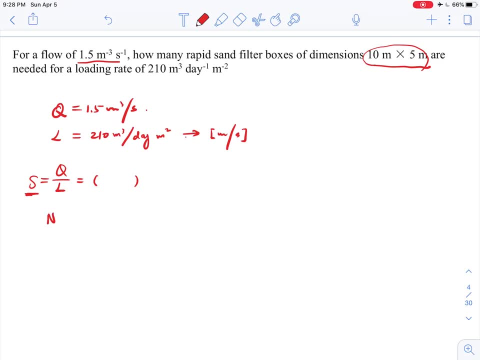 Right? So, basically, if you want to calculate what is the number of these sand filter boxes, then you need to further divide this S by the- basically each the surface area of each sand filter box, Right? So I think all of you got the correct answer for this step. 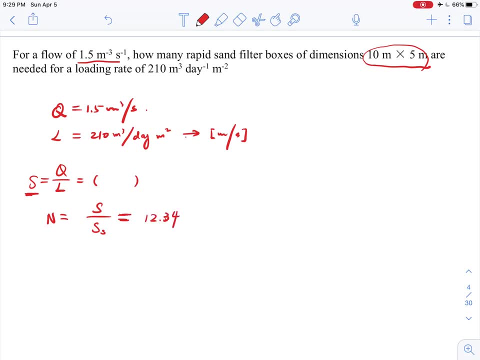 which is 12.34.. Okay, So now we have a decision to make, Right? So if it's 12.34,, then we can either choose 12.. We can choose 13,, 14.. Right, So I think all of you are trying to decide among these three. 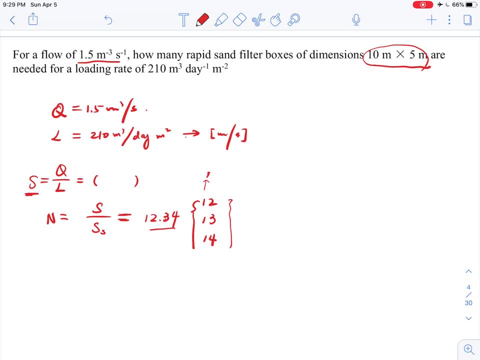 I didn't see that people choose one here because one is too much Different from the 12.34.. Okay, So we mentioned in the class and also in the review session that when we're trying to design the rapid sand filter boxes, people will always prefer even number of filter boxes because that's easier for the construction. 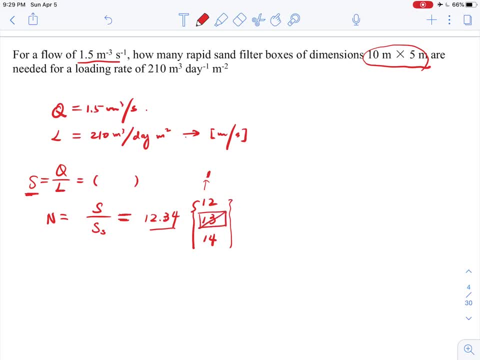 So, based on that, we can rule out the choice of 13 here. So it's either 12, or 14.. Okay, So I can tell that why some of you try to use 14 here? because here we're trying to make the system safer. 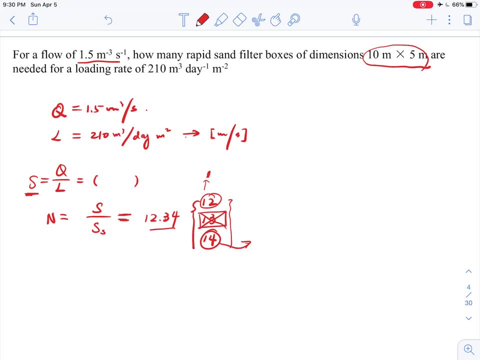 Right, If we have more sand filter boxes, then that's going to make this whole system more stable, because in this way, the loading rate is always below this required loading rate, Right? So why can't we choose that? So it turns out that we have to calculate this new loading rate and compare to that of the maximum loading rate of a sand filter box. 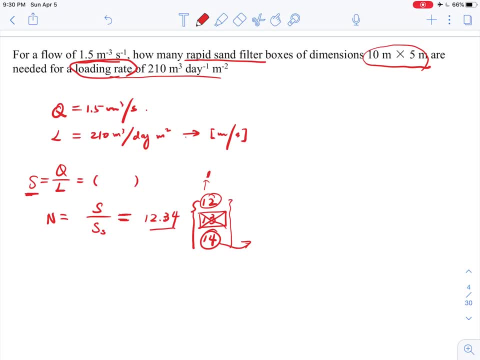 So we mentioned in the class that the maximum loading rate for this rapid sand filter boxes is 235 meter cube per day per meter square. Okay, So if we can design a system which has the loading rate below this value, then we're safe. 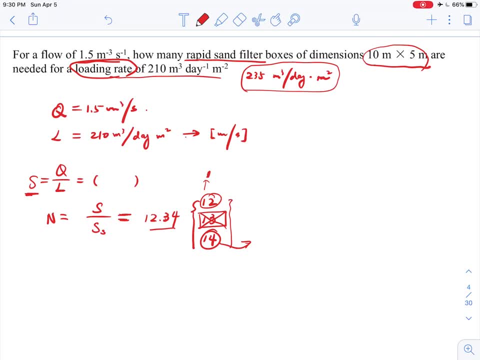 We don't have to create more sand filter boxes just to playing safe here, because you see that this problem is tries to design. this system has a loading rate of 210.. Right, So there are still some room between 210 and 235 here. 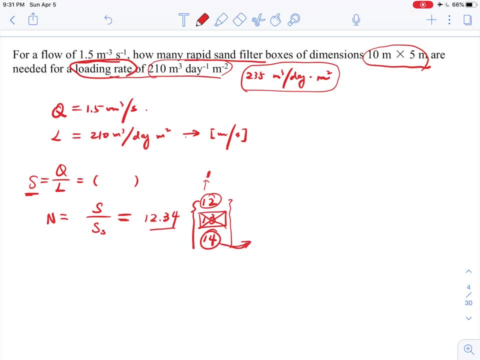 So we know that 14 for sure will work, but maybe we can save money By building 12 numbers of the sand filter boxes. I think some of you also directly get to the 12, because 12.13 is close to 12.. 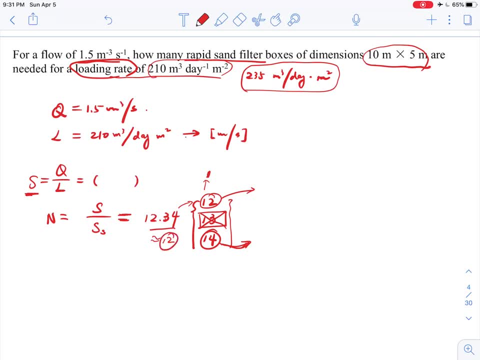 Right, You got the answer, but that is not the end of the problem yet, because you have to re-evaluate this loading rate or the actual loading rate. So how do we calculate this actual loading rate? So we can calculate that By dividing the total flow rate by the surface area, or the total surface area. 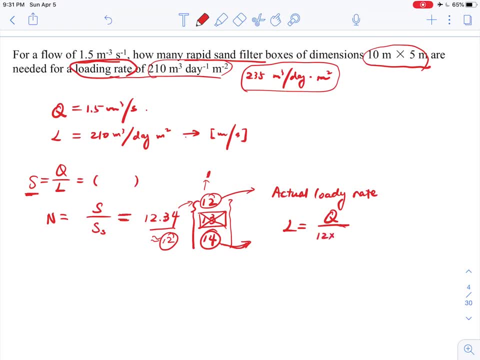 So we can use 12.. There are 12 sand filter boxes, Right? And then we know that the surface area of each one is 10 multiplied by 5.. Okay, So basically, if you convert that into the loading rate, meter cube per day per meter square. 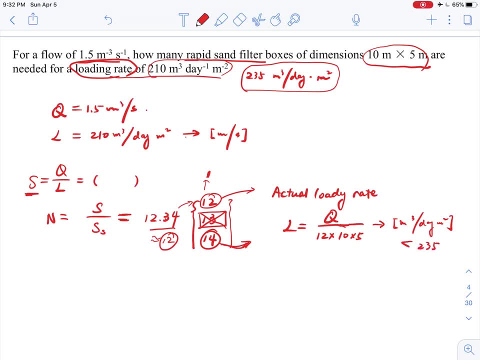 you can find that actually this value is smaller than 225. Okay, So if it's smaller than 235, it means that we're okay with 12 number of 12 numbers of the rapid sand filter boxes. Okay, So you can see that, if you directly get this answer here, 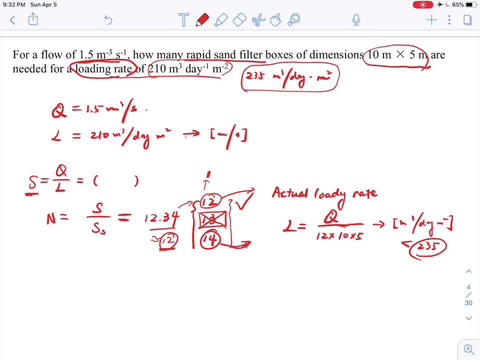 you may be lucky that, But since you didn't compare this flow rate, I deducted one point here. But if you got other answers- let's say 13 or 14, I deducted two points because on one hand, the answer is wrong. 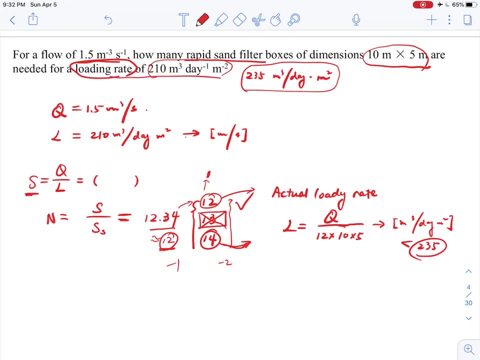 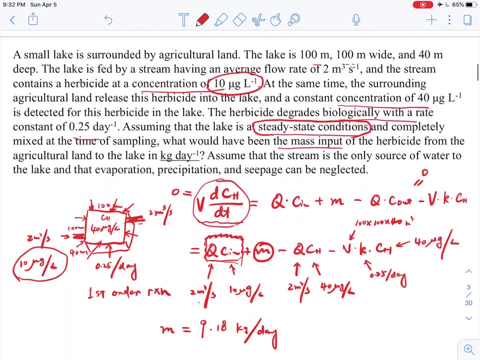 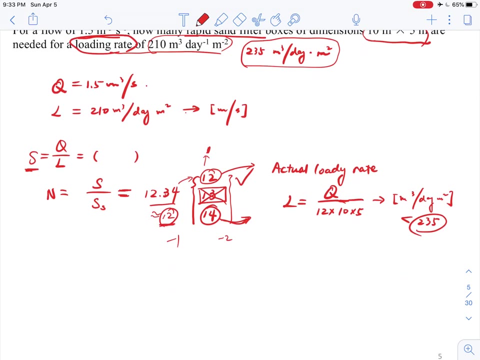 And also you didn't compare the loading rate of the system. Okay, So I think that's all for the common mistakes for this exam. two: I think as we get further into the design problems of this class, we're becoming more engineering based. 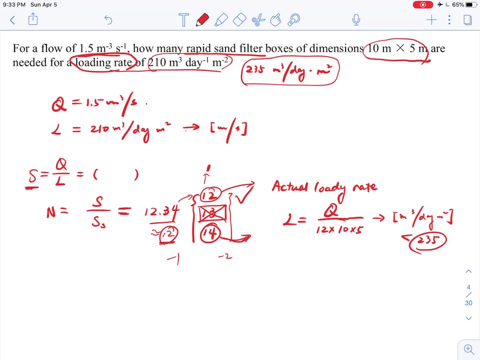 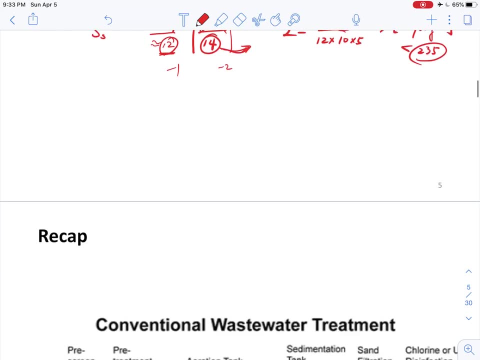 And I'm pretty sure that you guys like this more straightforward way of designing systems here. Okay, So for this class, we're going to continue on the wastewater treatment, So let's do a quick recap of our last class. So, last class. 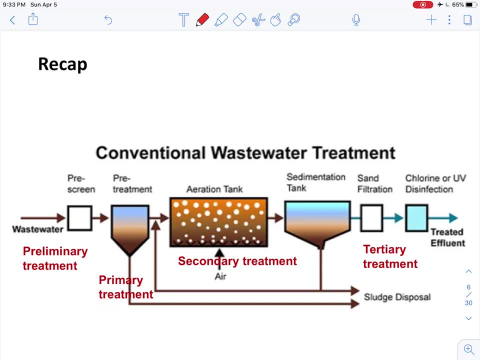 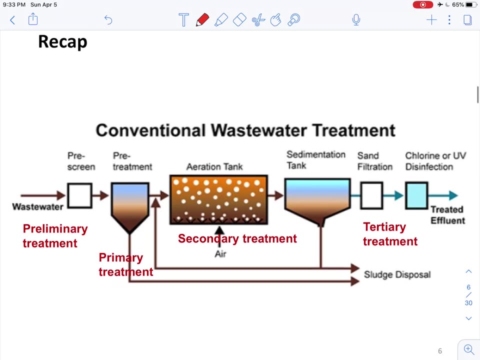 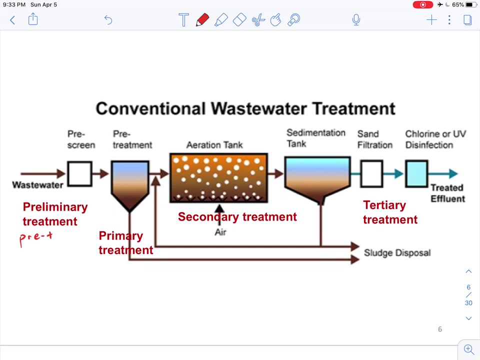 we did an introduction of the wastewater treatment systems right. We mentioned that there are multiple types of the isolated or small scale wastewater treatment And there's also industrial or municipal wastewater treatment process. So we mentioned that there are multiple treatment processes. There can be a preliminary treatment or we call that pretreatment. 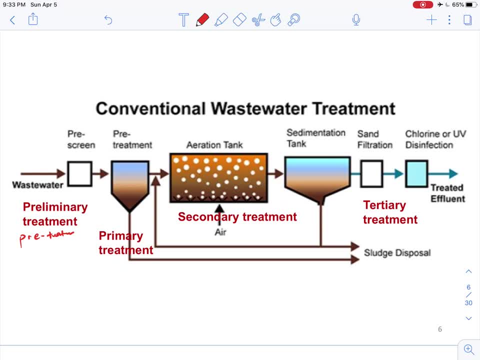 Right. There's also primary treatment. So basically the pretreatment will remove the larger solids that's in the wastewater. So there's also a primary treatment. So the primary treatment will further remove the solids that's in the wastewater And that is based on the concept of the sedimentation basin. 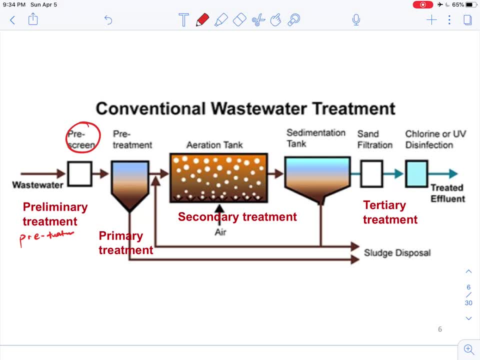 Okay, So we mentioned that the federal requirements or federal standards requires that all of the wastewater have to go through this secondary treatment. People will use the secondary treatment basically to introduce some biological microorganisms in the water to further lower the BOD. Okay, 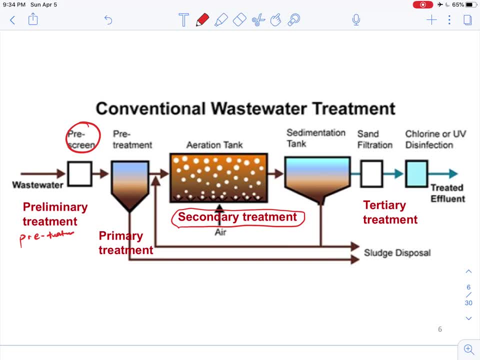 So after the aeration tank there can also be a second sedimentation tank, But both of these are categorized as the secondary treatment. So after that, after the secondary treatment, there can be a tertiary treatment. We can further filter the water or disinfect the water if the water is being reused. 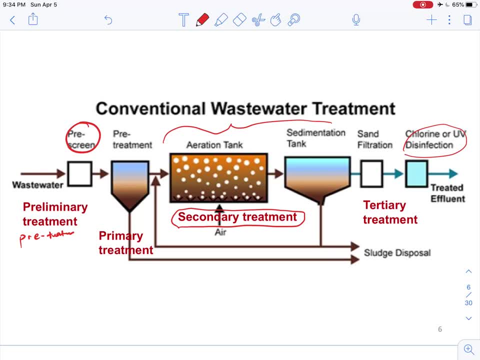 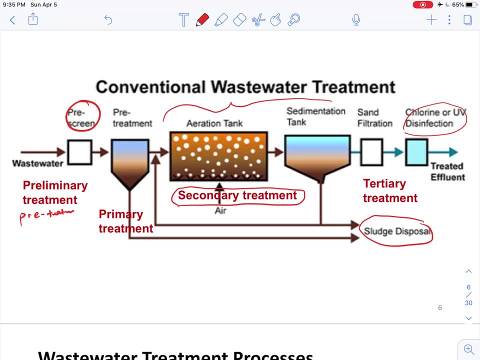 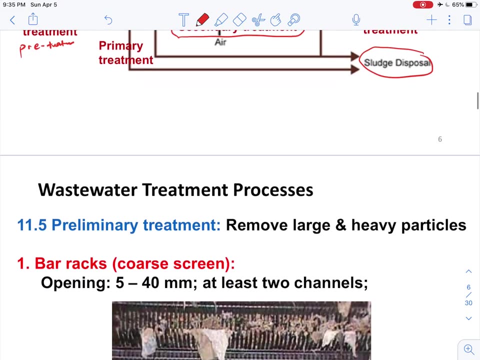 Right, So also mentioned that during these treatment processes we're generating a lot of sludge. Right, We have to process the solid waste properly. So here in this class we're going to go into the details of each step of this treatment process. 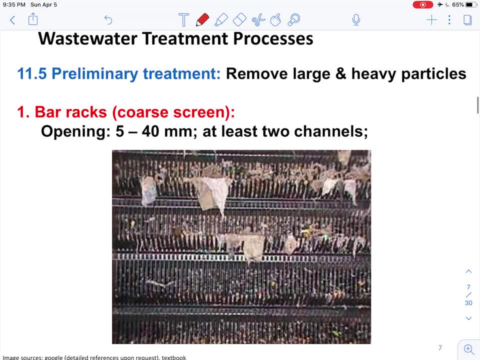 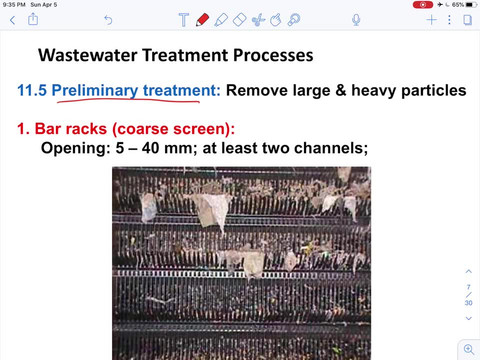 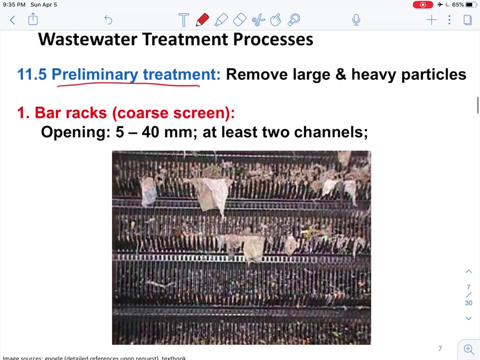 Okay, So the first one is the bar racks. So basically the bar racks are a part of the preliminary treatment or the pretreatment. So the goal is to remove the large and heavy particles. So, as you can see from the names, the bar racks are basically racks that can remove these larger solids here. 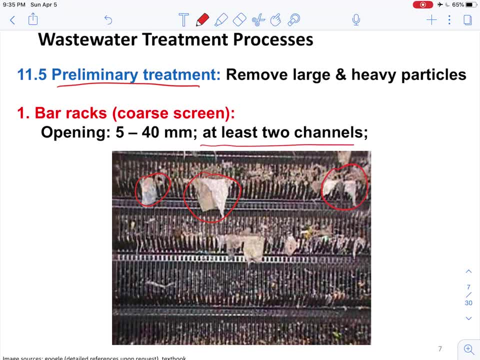 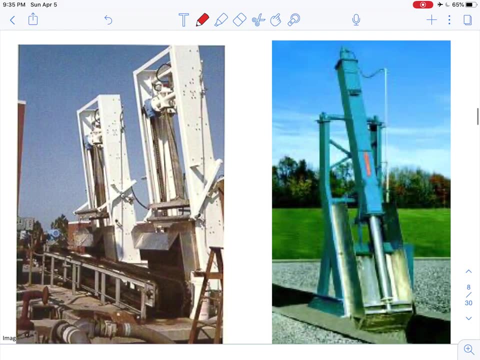 Right, Okay. And also people will design at least two channels here, mainly because if one channel is one of the bar is being pulled up for cleaning, we still want the other one to be in line to further clean the water there. So here you can see the real pictures of the real geometry of these bar racks. 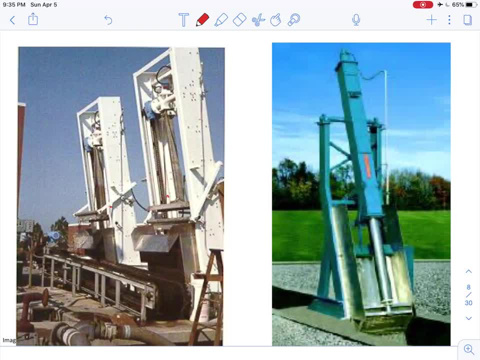 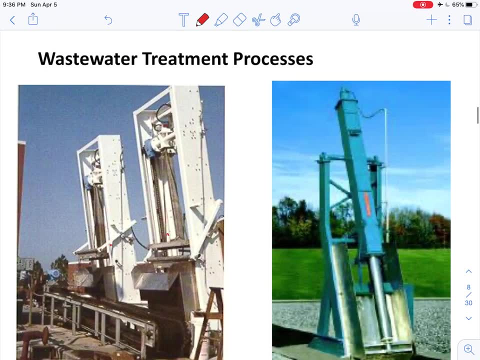 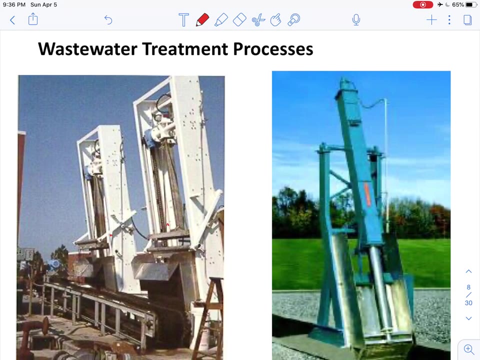 And you see that there are multiples of them. So here it's just showing one of them, but I'm sure that there's another one sitting beside it somewhere else. Okay, So people will typically use multiples of them or at least two channels to guarantee that there's a room when we are trying to clean these bar racks. 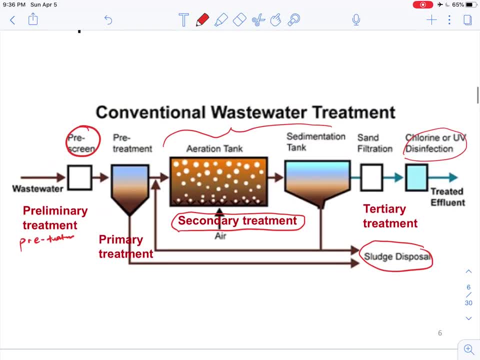 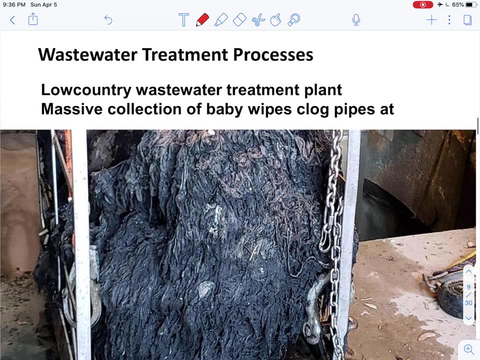 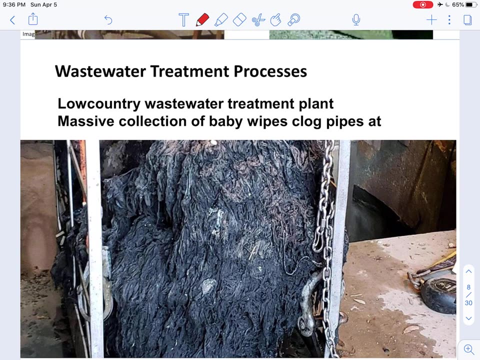 So we don't want all of these solids to go into the further downstream treatments here. Okay, So bar racks can be a direct way of removing larger solids, So here I'm showing some pictures of these solids that's being collected by the wastewater treatment plant. 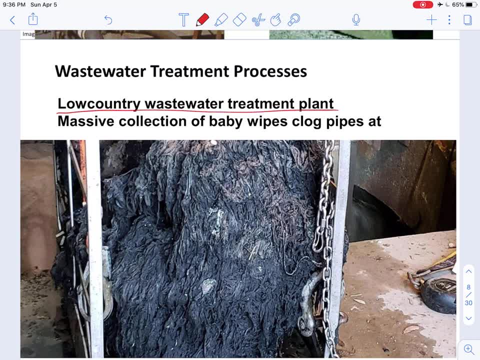 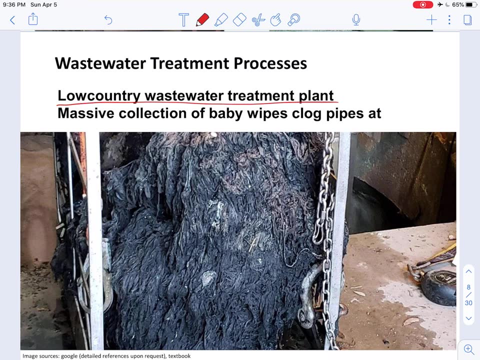 So this is showing a specific wastewater treatment plant And, as you can see, actually a large proportion, or the large proportion of these solids are baby wipes. Okay, So people thought that the baby wipes can be flushable, but they're not, Okay. 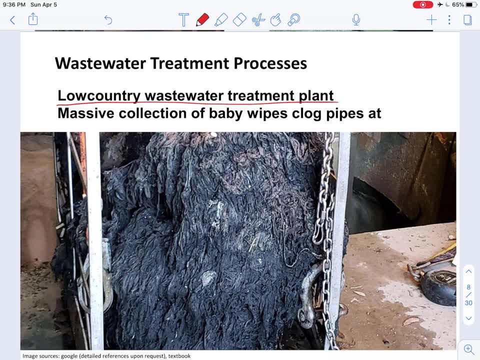 So, although it's not clogging the toilet right, but once they get into the sewage, there's no way that the baby wipes can decompose by itself. Okay, So that's why I think nowadays people design the new baby wipes that can. 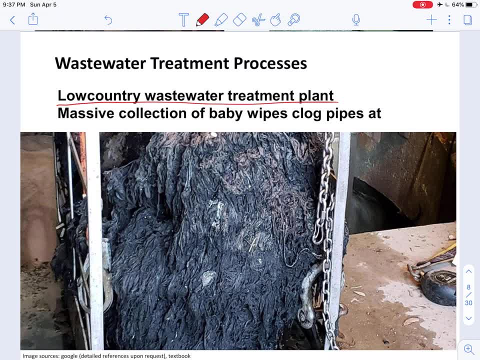 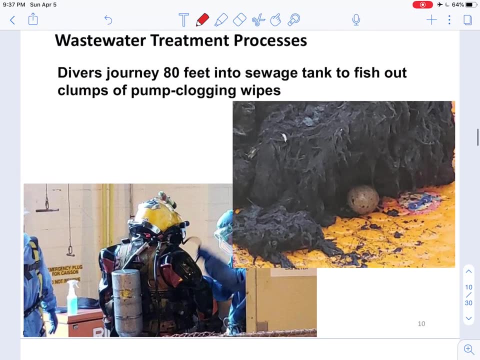 they call them flushable right. So basically those are safer for the water treatment plant So they can get decomposed by the microorganism in the water, so that they won't clog these water treatment systems. Okay, So here are some. 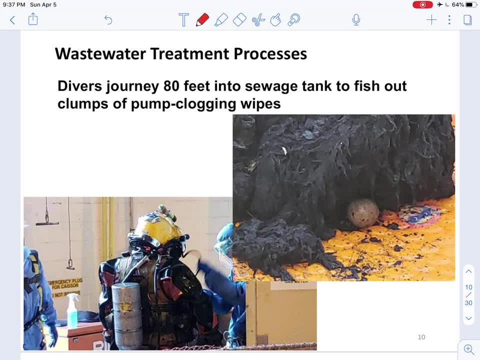 also some other pictures. So basically, once we get a massive amount of these solids here, once they really clog this sewage system or the wastewater treatment system, we have to send people down into these wastewater to collect these, because there's no way we can easily take these solids out. 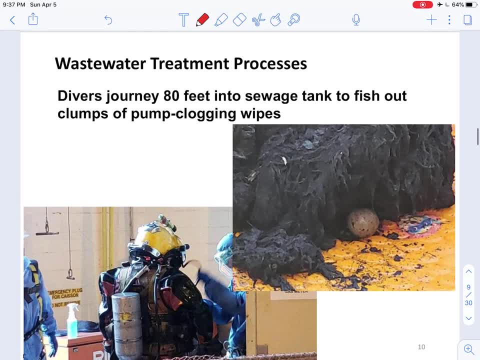 So basically, this is showing that divers will dive 80 feet into the sewage tank to fish out these clumps. Okay, So just for the benefit of these water treatment systems, we have to ask the workers or the who are on the frontline to guarantee that the water is safe to emit into the environment. 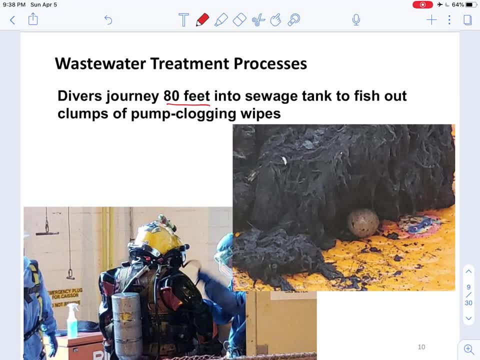 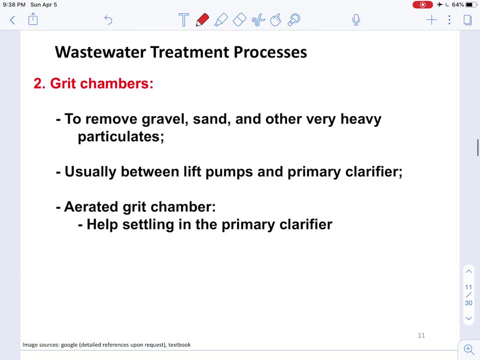 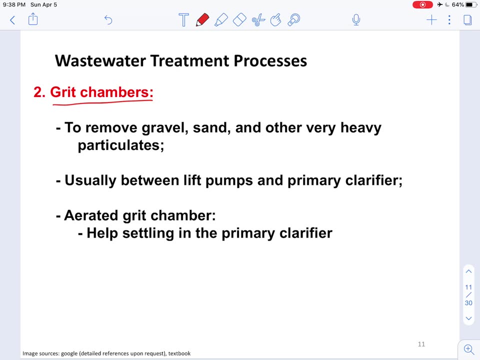 So please reduce the amount of solids in the water so that we're seeing less of these cloggings happening in the wastewater treatment plant. Okay, So that is a bar racks, and people also will use the grit chambers. Actually, the grit chambers are more commonly used in the pretreatment. 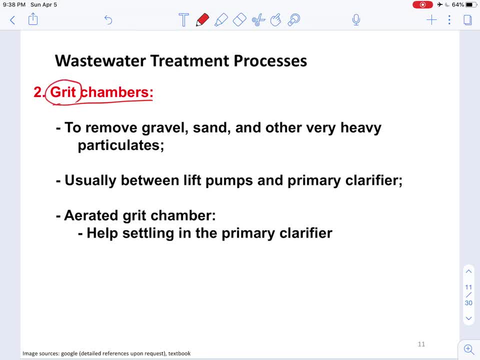 So here the grit just means particles. Okay, So they can be gravel, sand and other very heavy particulates. So you can see that people use different terms to describe basically the same thing there. Right, So for the drinking water system. 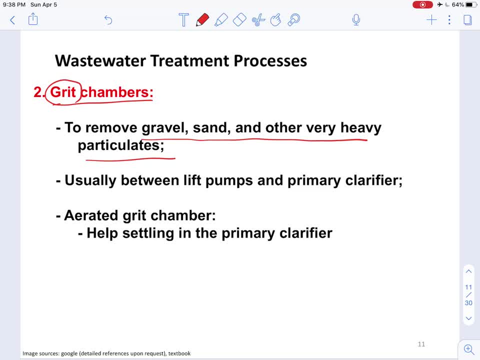 we call these heavy particles, We call these colloids, Right, So those are particles. And here in the wastewater treatment we call these particles as grit. Okay, So the grit chambers are typically between the lift pump, so lift pumps are at the beginning of this wastewater treatment plant. 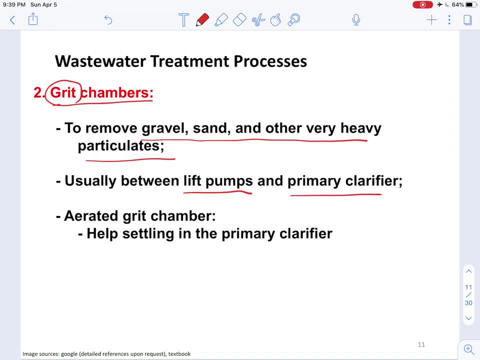 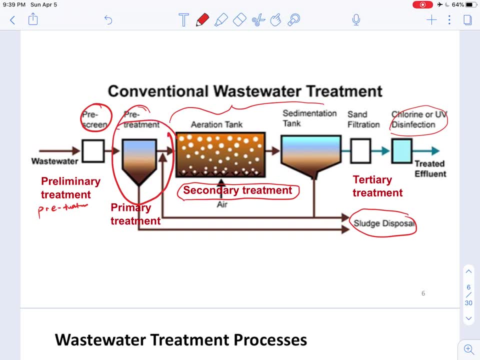 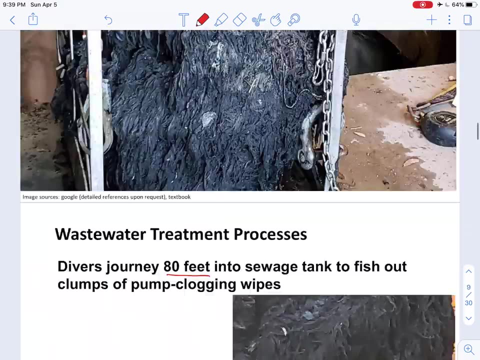 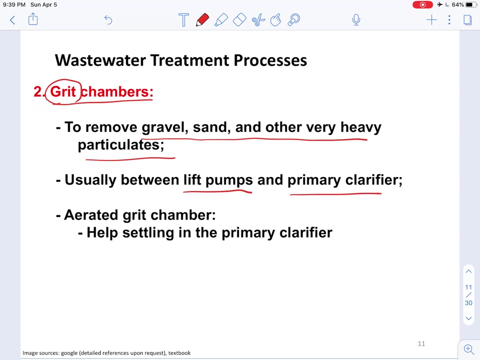 It's between the lift pump and also the primary clarifier. So the primary clarifier is here. Okay, So that is the primary treatment process of the wastewater treatment plant. Okay, So we'll use the grit chamber somewhere here. So what the grit chamber does is: 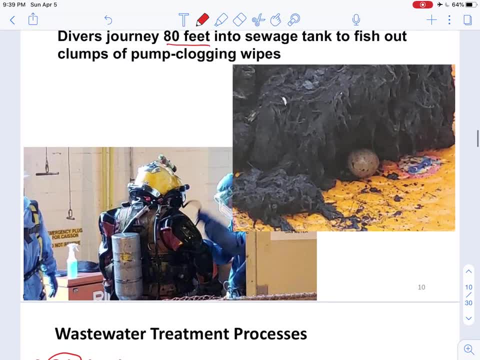 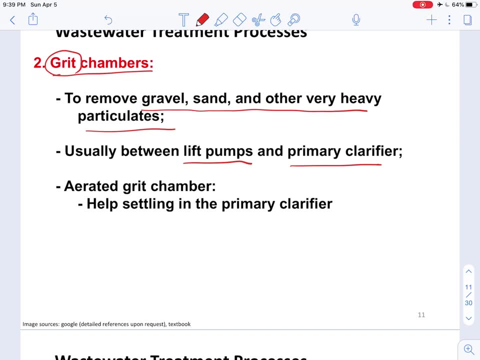 it removes these particles from the wastewater. So the bar racks removes larger chunks of solids, Right. So the grit chamber will remove particles in the middle size that are still in the water, but relatively larger. Okay. So people design these aerated grit chamber. 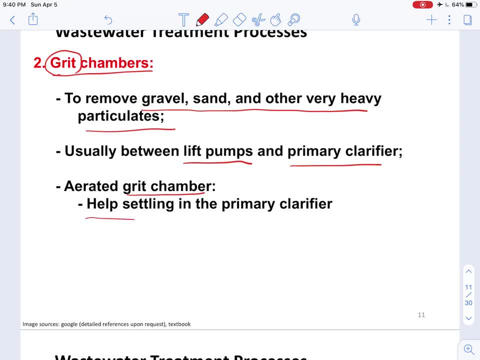 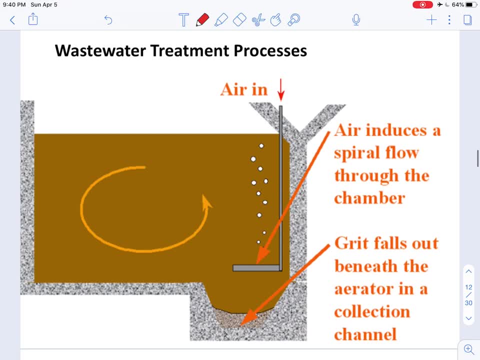 So these will basically remove those larger particles and further help the particle settling in the primary clarifier. Okay, So the mechanism of these, of these aerated grit chamber, is that when we have these ducts of water going through. So let's say that here. 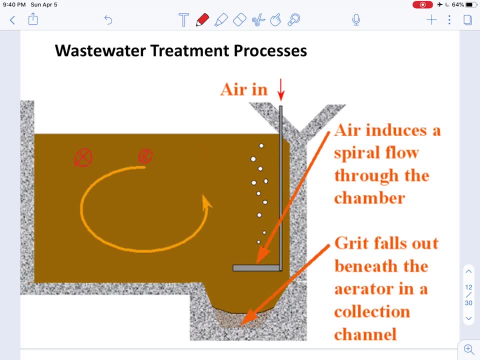 let's imagine water is going inside into this screen here, Okay, So what happens is that we're going to introduce air into the system, So the air is going to. I think this is drawing the wrong direction. So the air is going to. 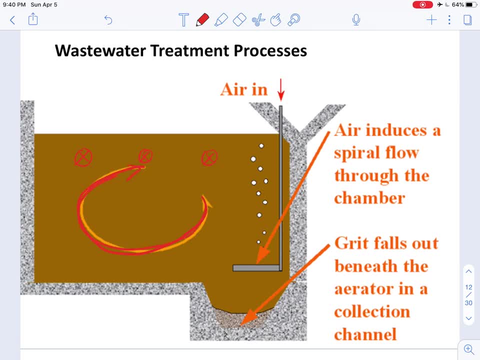 is going to go this way, Okay, So that's going to make the water to rotate, or to basically spin here. So let's say there are solid particles or very heavy particles in the water. So what's going to happen? So, to maintain the rotation of the particles. 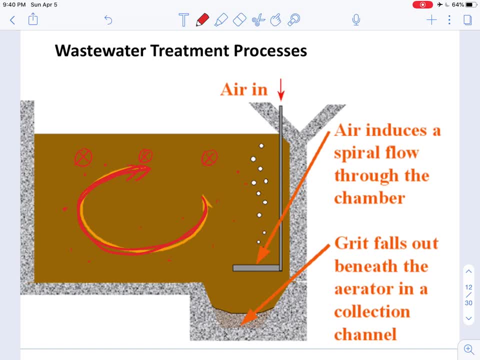 they need centrifugal force, Right, But here they don't have any. So what? that means that the larger particles are just going to get spinned out, Right. So they're going to move this way, They're going to spin out. 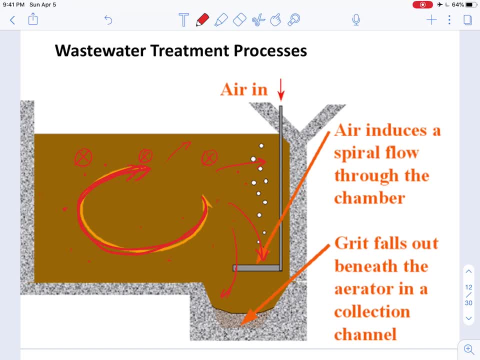 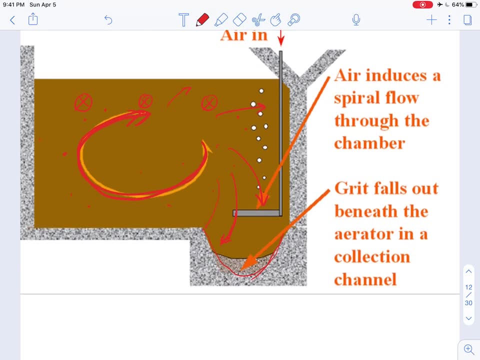 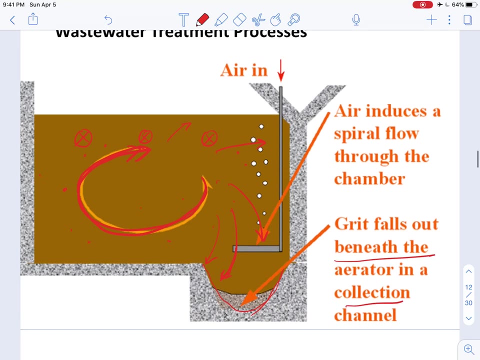 So by spinning these particles out, we have a collector here. So basically, this is a dip that's in the flow channel here. The particles will just get collected in the channel and then falls out beneath the aerator and get collected in this channel here. 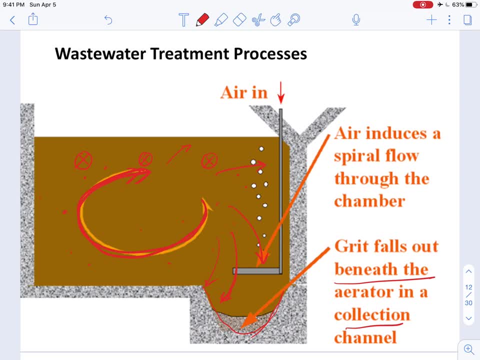 So you can see that this system works like a cyclone or a tornado here, Right, So people were actually- people were actually using these designs in many types of pollution treatment. You can see that here is treating the water quality Actually in the air pollution. 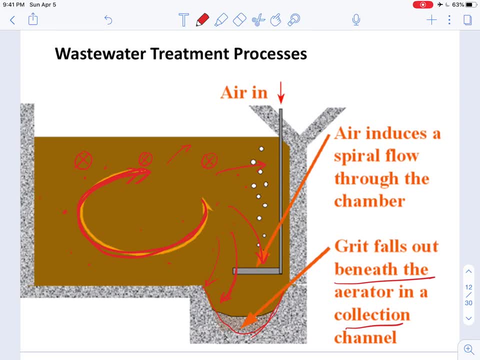 which is at the- maybe next month we're talking, we're talking about next few classes when we're talking about the air pollution, And we'll also talk about these systems. So that system is specifically called a cyclone. Okay, So it's using a similar technology. 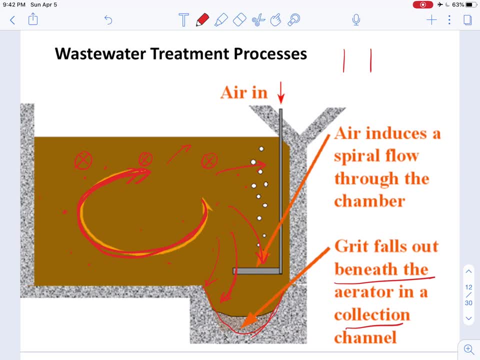 So basically you have a cylinder Right, So the air is being introduced from the side of it, And then you're having these vortex or rotation movement here, So the larger particles will just get spin out and then get collected onto the walls of the cyclone. 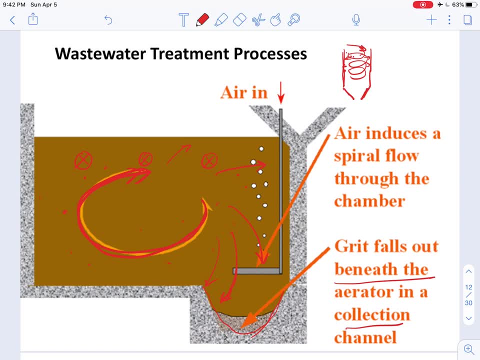 And then at the bottom we have a dust collector Right, So the particles, after they hit the wall, they will fall down and then we can purify the water and get rid of the particles there. Okay, So that system is called a cyclone. 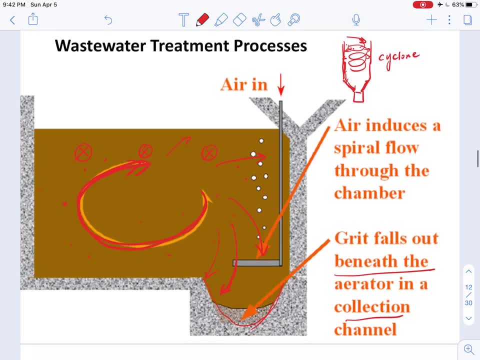 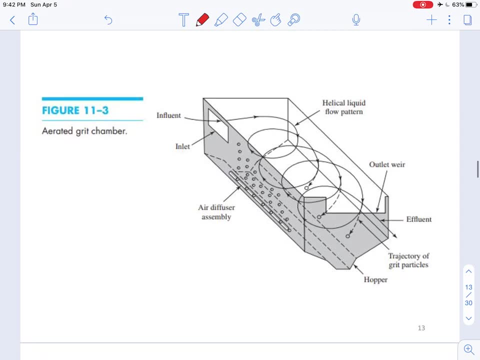 So it's using a similar mechanism as the aerated grit grit chamber. Okay, So here is showing another picture of this grit chamber- aerated grit chamber. You can see that we have the inflow coming in Right. We also have the air diffuser. 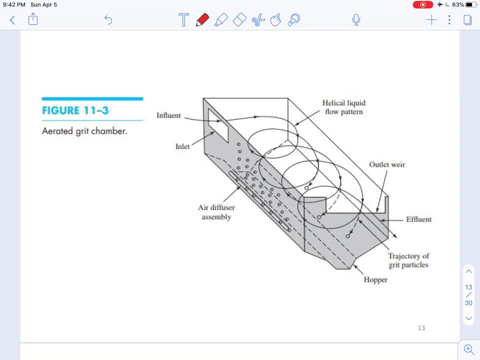 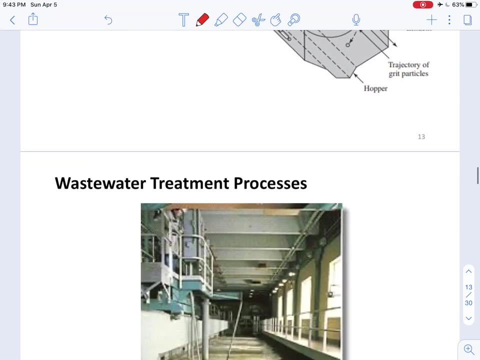 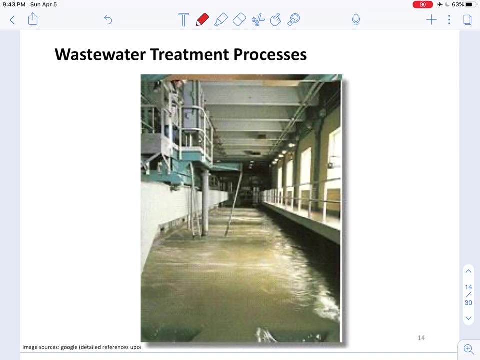 Right, So we're creating these rotational movement of the water, So basically, we can remove these larger particles and then get them collected in the hopper here. Okay, So this is showing how an actual system or actual aerated grit chamber looks like. 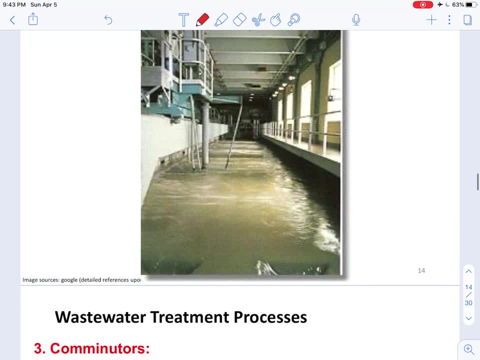 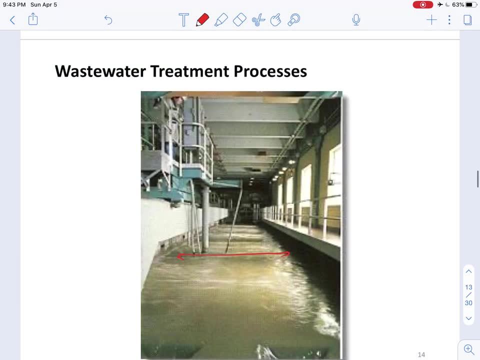 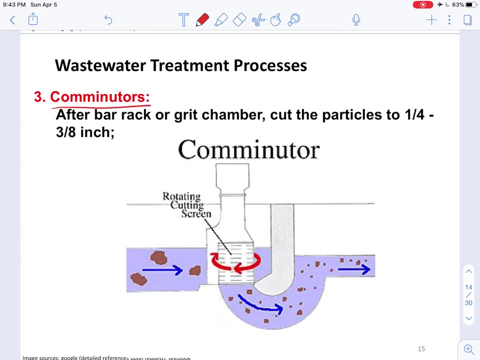 So they are typically in a larger scale. You can see that this channel here is probably what? four meters wide. Okay, So for the pretreatment, people will also use the calming neuters. So what the calming neuter does is it's going to grind the particles. 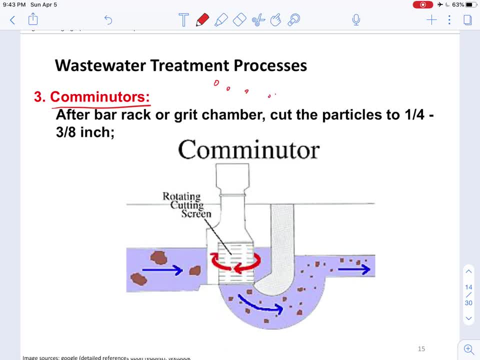 the remaining particles into small pieces of particles. So basically, after bar rack or the grit chamber, they will cut the particles into quarter or three eighths inch. Okay, So those are going to get into smaller sizes. So what happens is that the calming neuter are going to 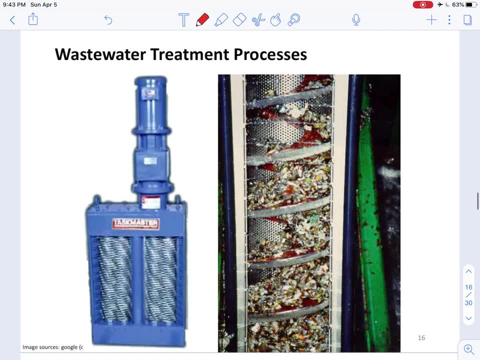 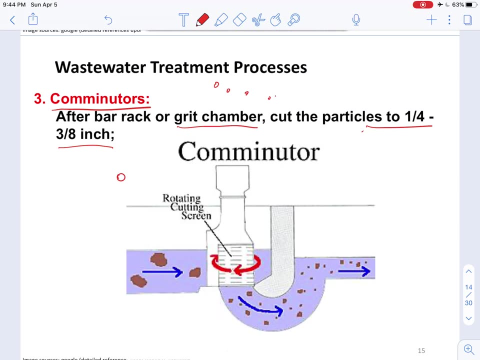 cut these species and actually they look like this. So you have these two cutters here and then they just rotate, So to grind those particles into smaller pieces And after they get into these more uniform sizes here, we can introduce them into the primary treatment. 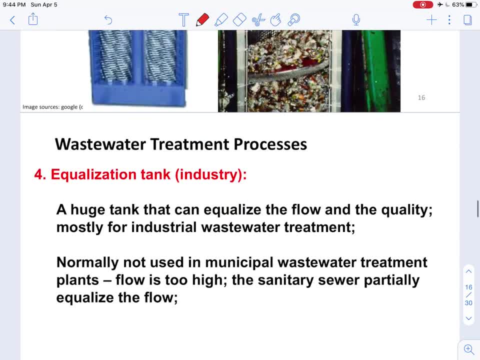 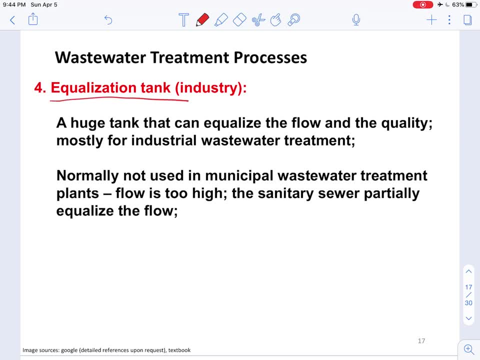 or the primary clarifier to remove these particles. Okay, So for the pretreatment we also have a system called the equalization tank, So the name might seem a little bit confusing here, but what that really means is that we need a tank to store the wastewater. 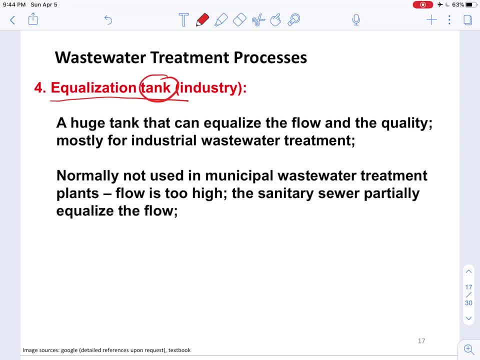 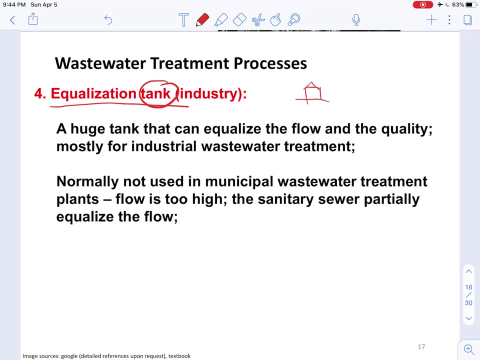 So basically that will prepare the system with different types of flow rate. So for example, if we have a type of industry right, So we introduce a slaughterhouse in our last class. So for those industries there I'm pretty sure that the demand or the supply is really depending on. 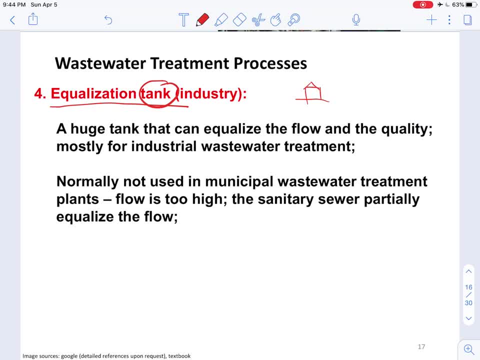 the time of day. So during the daytime we may generate a lot of wastewater, and during night there's no wastewater. Okay So, but we want the wastewater treatment to be continuously running, because if we stop it and then keep it running again, 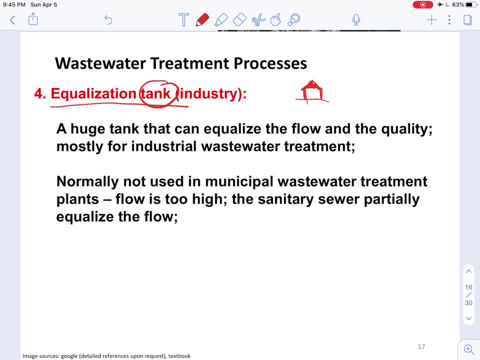 then that's going to cost a lot of maintenance process, right? So what happens is that we're going to create a tank right To store these extra or excess wastewater, right, And then we can introduce them into the treatment process. So what happens during the daytime is that the treatment is still 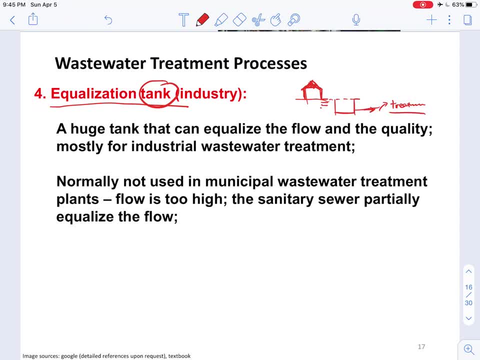 processing water, but it's at a lower flow rate. It doesn't compare, cannot compare to the larger flow rate during the daytime processing. So the extra or the excess water are just going to get stored in this equalization tank. Okay, So after the processes are finished during the day, 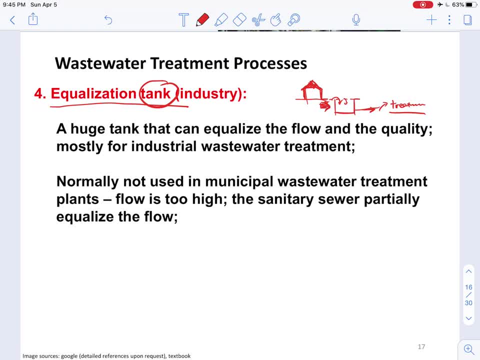 right, There's no wastewater generating out, So we can further consume these existing wastewater in the tank to treat them with the water treatment facilities here. Okay, So basically the equalization tank is a huge tank that can equalize the flow and the quality. 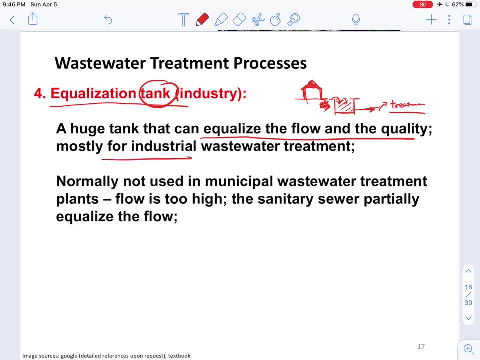 And also it's mostly used for industrial wastewater treatment, because for the municipal wastewater, they are typically generated at a relatively constant flow rate. Okay, So for the municipal wastewater, on one hand it's because the flow is too high, So we cannot easily find a tank that can accommodate this much of a flow. 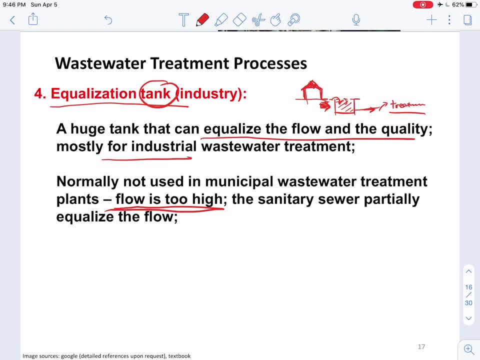 rate, or this much of a flow, And also for the municipal wastewater treatment plant. we also have this sanitary sewer, which can partially act as an equalization tank there. Okay, So we have those larger systems in the sewage system that can store these. 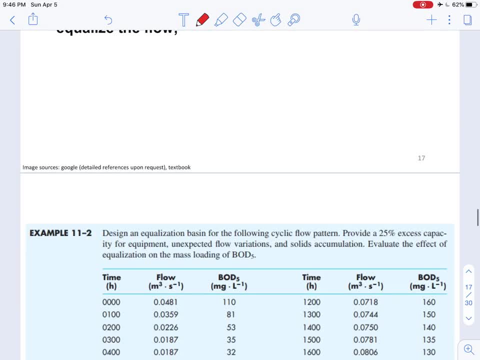 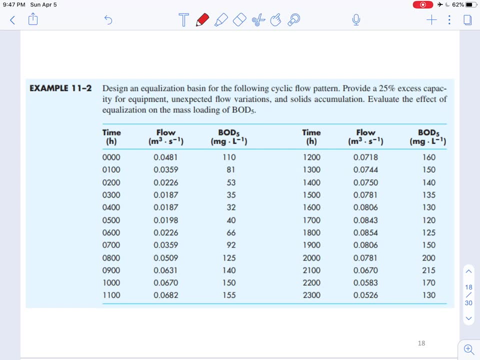 excess uh wastewater. Okay, So uh, in your textbook you can find a uh example problems that is trying to let you design a equalization basin, equalization tank for removing the um, so basically to collect these. 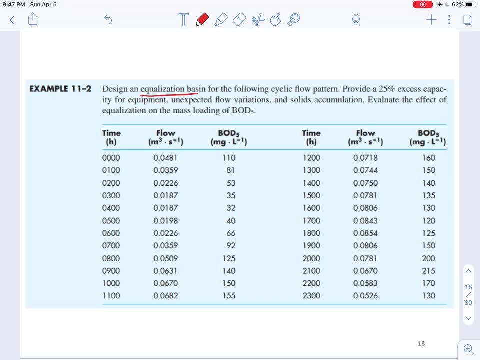 uh excess wastewater. So you can see that for this industry, um, at different times they're going to generate the flow at a different flow rates. right, You can see the highest flow rate is generated somewhere near uh what? 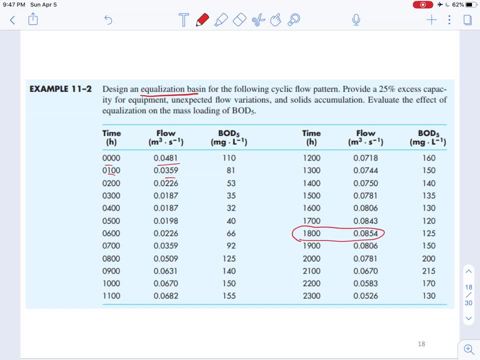 Somewhere near uh 6 pm. Okay, So that is time. that is the time you are generating um the most wastewater, And during the daytime the flow rate is relatively low. During early morning, the flow rate is relatively low. 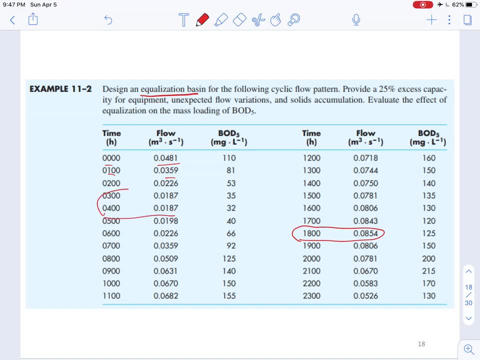 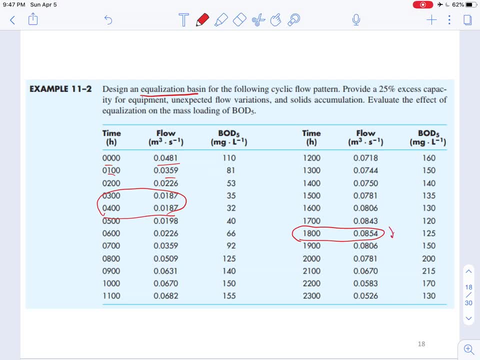 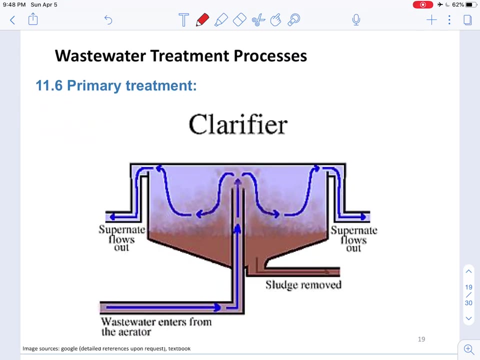 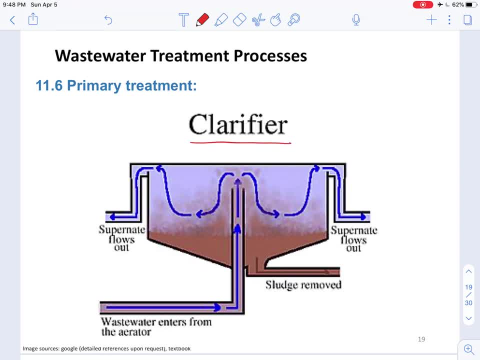 people will use the clarifier. Okay, so we'll also introduce these clarifiers in the drinking water treatment process. So for the wastewater treatment process, the clarifier is a very simple, um simple device, So it is just using the sedimentation or the settling of the particles to remove these. 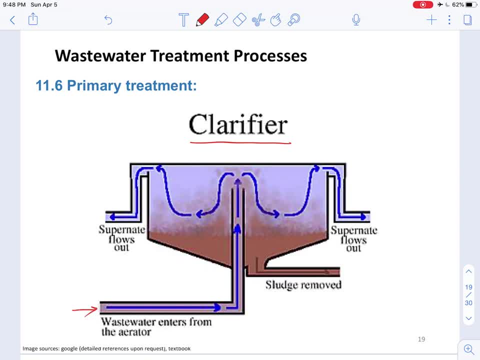 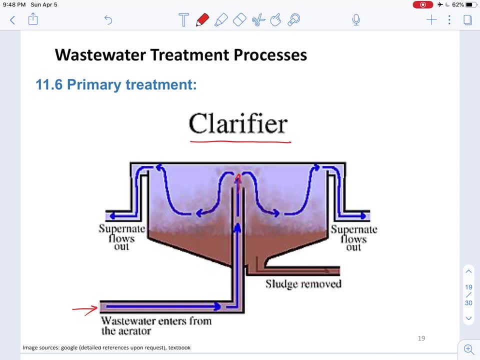 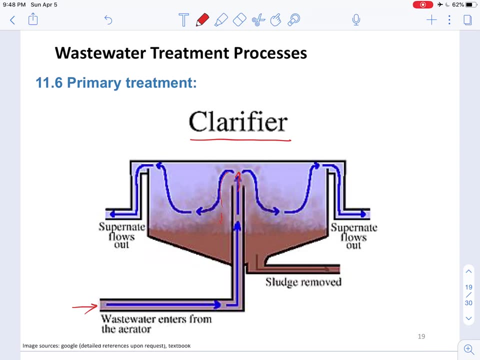 remaining solids. okay, So you can see that wastewater is being generated from, or being introduced from, the bottom, and then it's going to flush into the top, right, And then, because the solids have a gravitational force right, So they can get settled down into the base of the 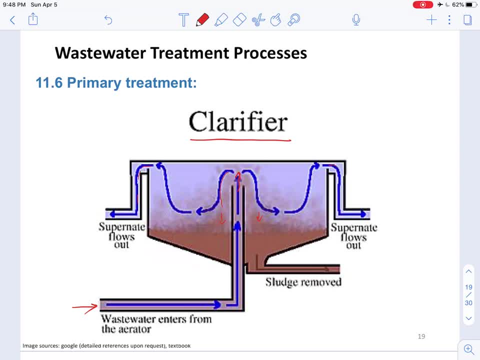 clarifier and then the water can further get collected from the outside. okay, So the clarifier just use the sedimentation. okay, So you can think of it as a sedimentation basin, but will have a different type of geometry or different name here. So we also introduced 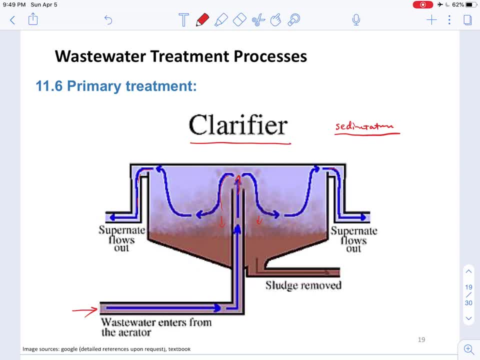 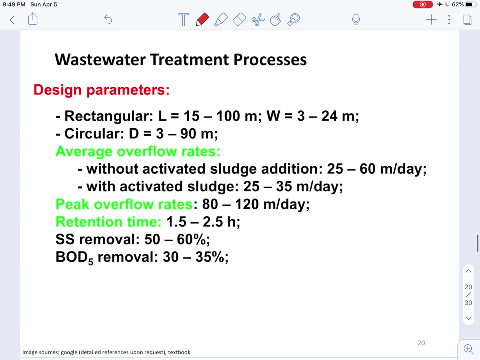 in the review problem of the exam. two: right. So for the sedimentation basin, what is the primary design parameter? That is, a surface overflow rate, right. So the same concept will apply here for the clarification of the wastewater in the system here. okay, So there. 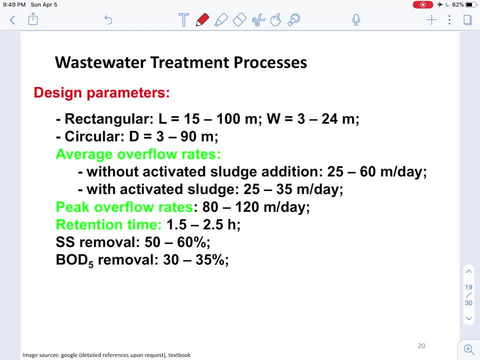 are a few design parameters for these primary clarifiers. So if we're designing a rectangular primary clarifier, we'll typically look into a length of 15 to 100 meters. The width is shorter right, 3 to 24 meters wide. If we're 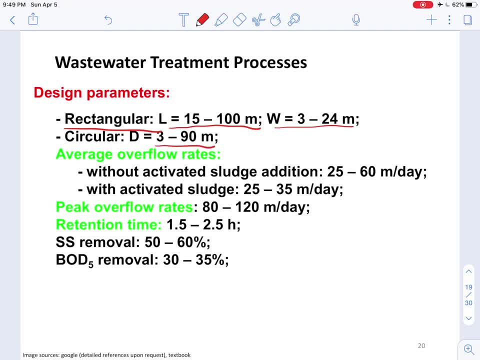 designing a circular one, then the diameter is between 3 to 90 meters, So you can see that this is a very large range here, right? So you can really. this is really depending on the flow rate of the wastewater we're trying to process. If the flow rate of the wastewater is very low, 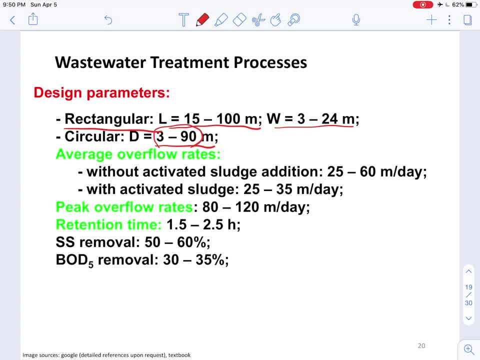 then we can just design smaller clarifiers to accommodate this wastewater. So the average overflow rate, which is talking about the sedimentation, right, So without the activated sludge which we'll introduce later here. So without the activated sludge the overflow rate is 25 to 6 meters per day. and if we're adding in the activated 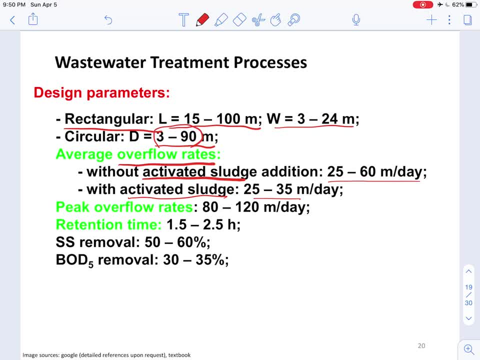 sludge is around 25 to 35 meters per day. So basically, with the activated sludge we're going okay. so by having a smaller overflow rate that means the residence time of the wastewater in the clarifier is going to be longer. the residence time. 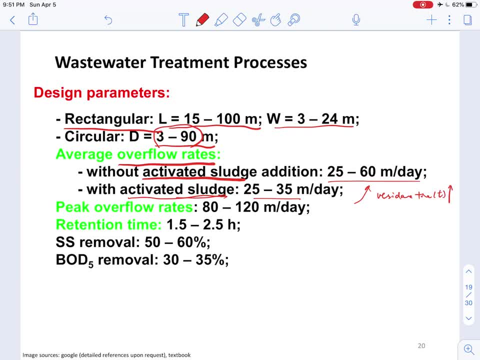 residence time or retention time or increase. okay, so the peak overflow rate is around 1880 to 120 meters per day and the retention time or the residence time is 1.5 to 2.5 hours. you can see that this is ready for a long time here. 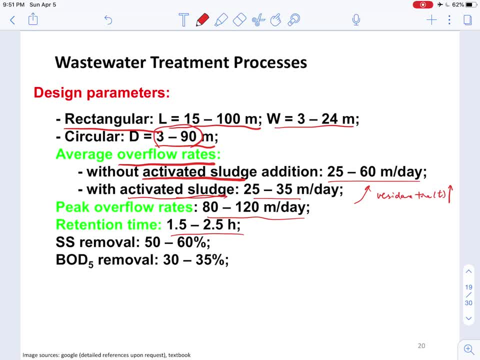 because we're trying to let these particles- quarter inch or 3, 8 inch wide solid particles- to settle down by themselves. okay, so the solids suspended solid removal for the primary clarifier is around 50 to 60 percent and the BOD5 removal is around 30 to 35 percent. okay, it really depends on. 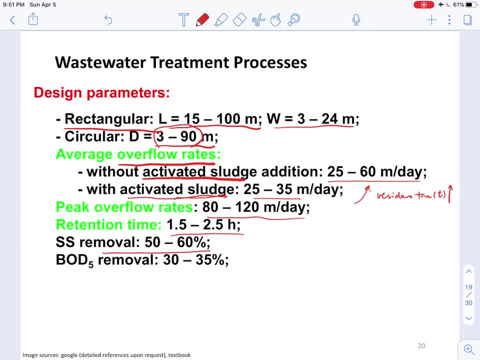 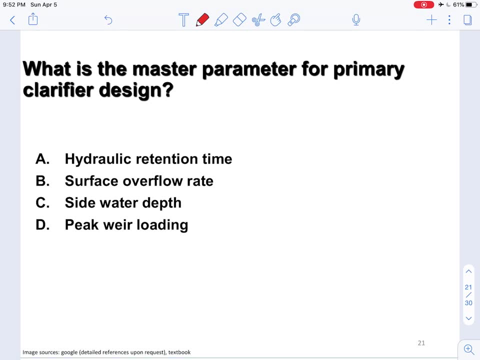 whether we have the activated sludge in the system or not. so the activated sludge are the microorganisms that can oxidize these organic materials, which can reduce the BOD5 in the water. so again we have this question: what is the master or principal parameter for the primary clarifier? 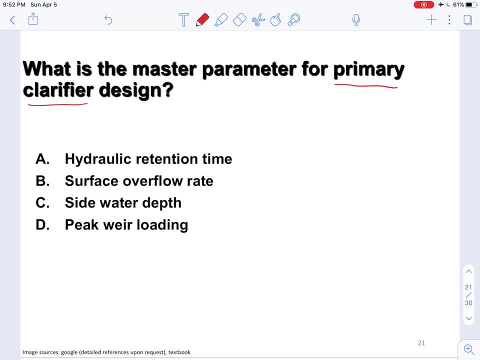 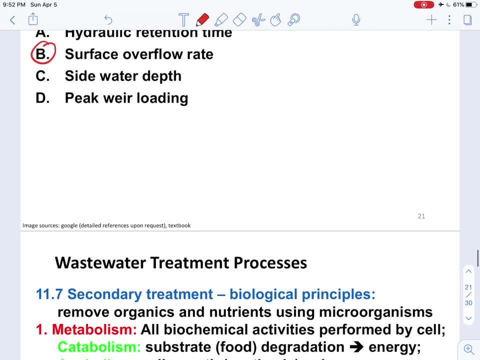 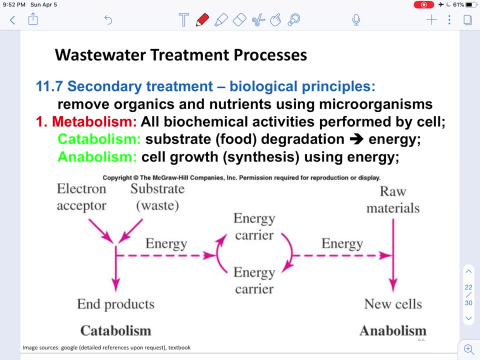 that I do not want to say yet. so some of the Pro emperorμ that the primary clarifier is similar to a sedimentation basin. so what answer should we choose? that should be b. we're talking about the surface overflow rate. okay, so that's all for the primary treatment process. so although we call them primary, but the mechanism? 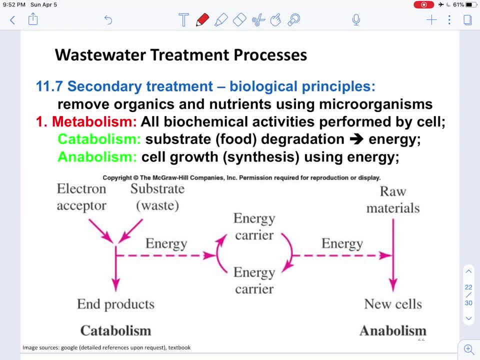 is really simple. so that's why federal requirements will require a secondary treatment to further purify the water, because we know that just by settling these solids it's not enough to remove the suspended solid and also the organics in the water system. okay, so the secondary treatment are basically using these biological principles, so we're using these. 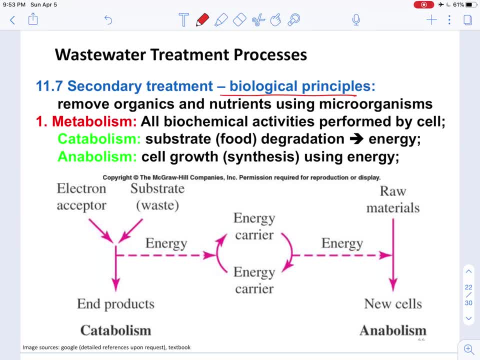 microorganisms to oxidize the organics in the wastewater, so they can remove the organics and the nutrients using these microorganisms. so we're talking about the metabolism, which is a process that the microorganisms conduct during this process and during this treatment. okay, so the metabolism is the um. basically it's defined as all the 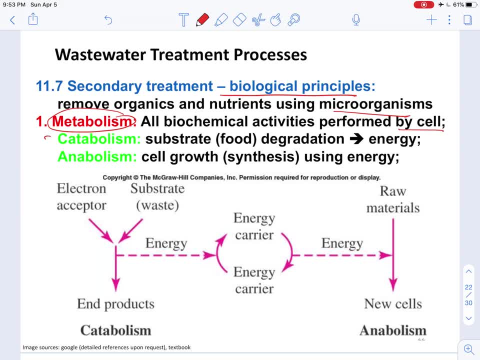 biochemical activities performed by the cell. so it can be further classified into the uh, catabolism and anabolism. so catabolism means basically that is, the consumption of the food and convert that into energy. okay, so this is the pure consumption of the organics. okay, so anabolism means cell growth. so this is basically generating more cells. okay. 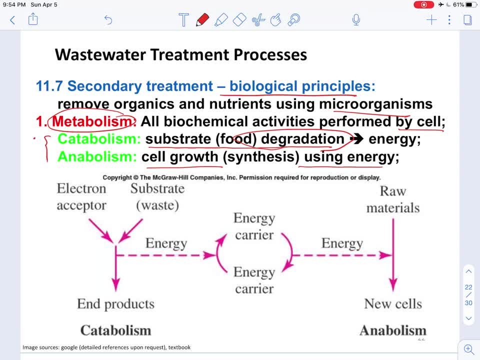 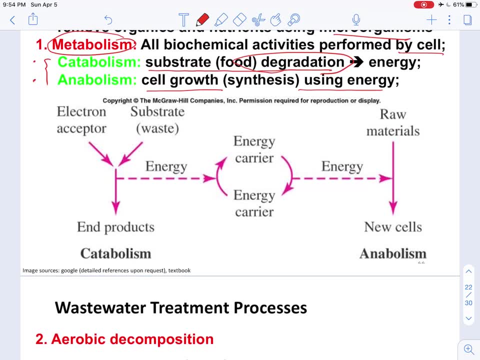 so one. so the major difference is that this one is just the system sustaining the cell itself, while this one is creating more cells. okay, this one is just sustaining the cell itself, while this one is creating new cells. so here is a very simple diagram that's showing the 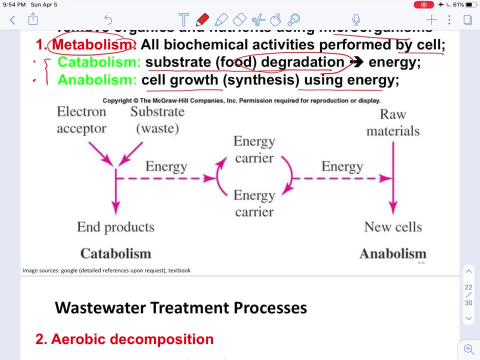 difference between the catabolism and anabolism. so the catabolism is just consuming the substrate or the waste right to generate these end products, so for example, carbon dioxide, water or other types of organics. but once we generate these energy, then they can convert into new energy and then produce. 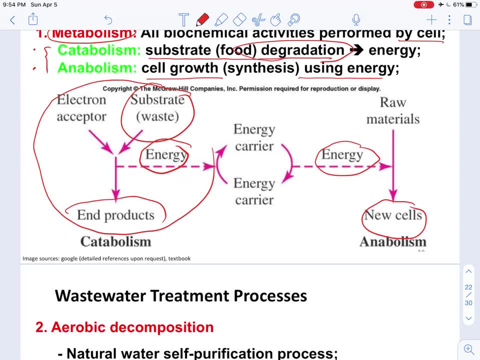 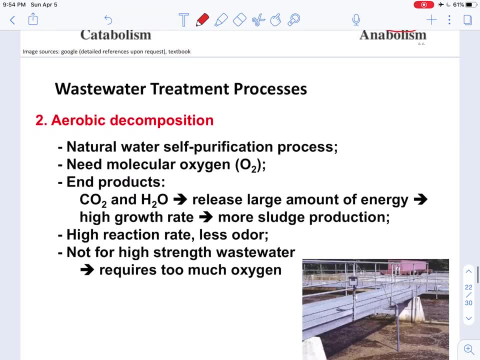 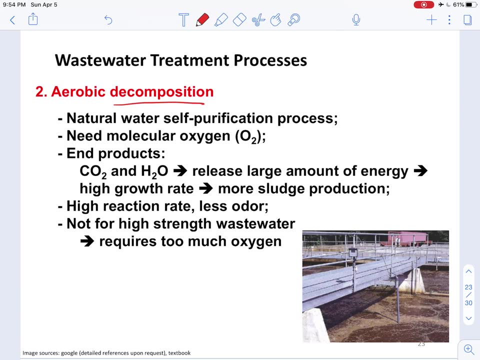 these cells. once the new cells are produced, we call this process as the anabolism. okay, so in terms of the biological treatment process, there are different types of decomposition processes. so there can be aerobic decomposition. so aerobic decomposition means the decomposition that needs oxygen as a feed. okay, so this is also the process that the natural water self. 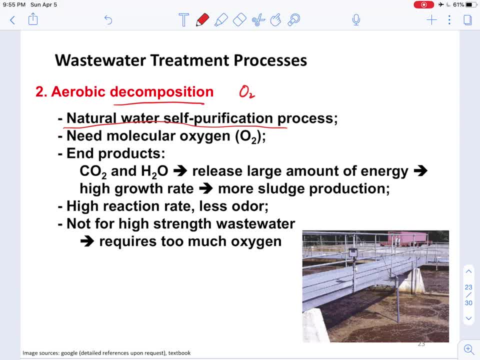 purify itself. so we introduced the deal sag curve right deals that curve will need. we're showing that curve there because the organics in the water to oxidize them they need oxygen and that to be pumped into the, into the river water, okay. so that need oxygen and basically that process is the aerobic decomposition. 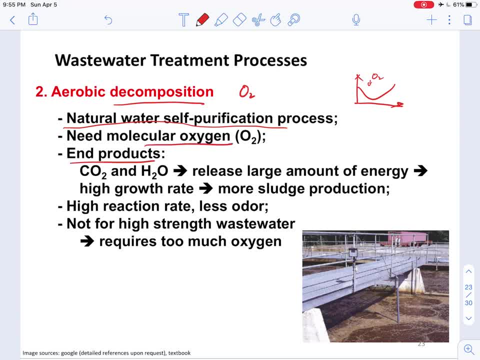 okay. so it needs molecular oxygen and, in terms of the end products, we can generate carbon dioxide and water, and one thing we need to notice is that for these aerobic decomposition process, they will release large amount of energy. so this is the major difference between the aerobic decomposition and other types of 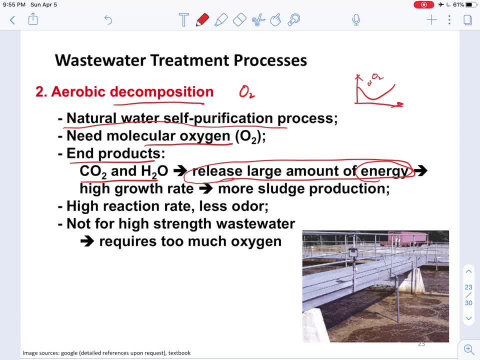 decomposition processes and because we produce a lot of these energy for these microorganisms, they're going to have a very high growth rate. if they have a high growth rate, then they are going to produce more sludge because we're generating more solid bacteria or microorganisms in the water. 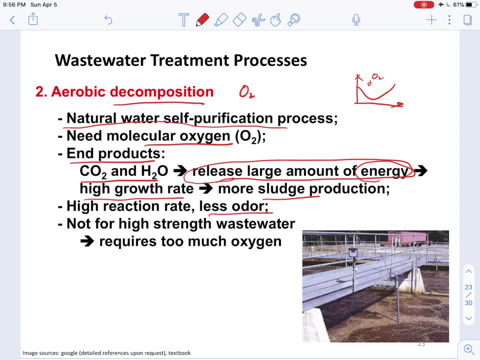 okay. so we have the higher reaction rate. that means there will be less odor, because the odors are typically organics that are also having a relatively low, relatively high volatility, so they can get vaporized and then form those, those odor, and also for aerobic decomposition those are. 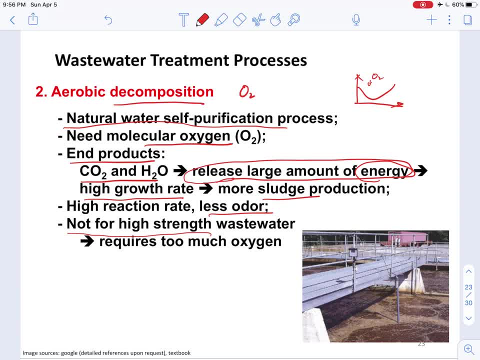 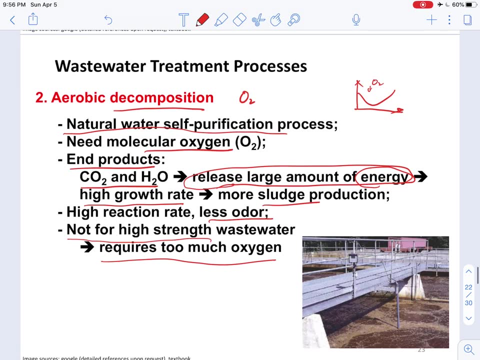 designed for, not designed for, high strains wastewater. so because if that's high strains wastewater, which means that it contains too much BOD, then it's going to require too much oxygen, which is not, which is not really suitable for these processes. so this is aerobic decomposition. so we also have the anoxic. 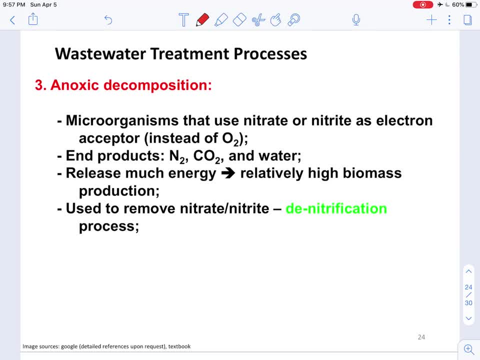 decomposition, which means that it's going to use less oxygen. okay, so, or no oxygen for certain types of oxygen, types of the microorganisms. so for these microorganisms, they use the nitrate or nitrite as the food at their energy source. okay, so they are going to produce. 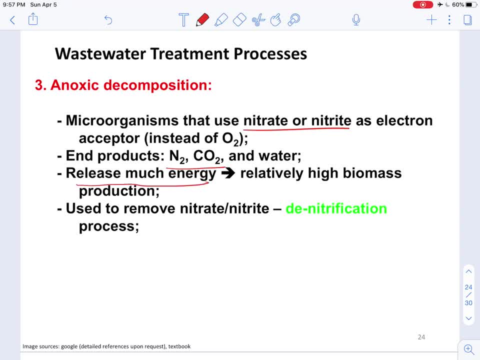 nitrogen, carbon dioxide and water, so they also release much energy, which means that they are going to generate more sludge, or hot record high biomass in the sludge there. and another advantage for these anoxic decomposition is that they can remove the nitrate, or nitrite. okay, so we call these process as the 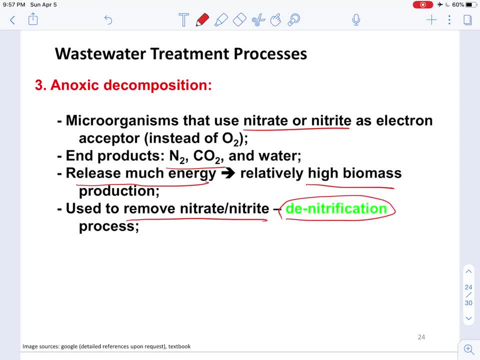 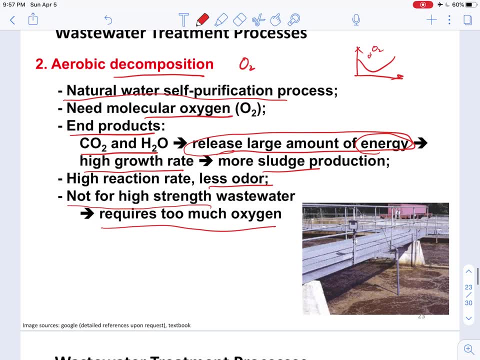 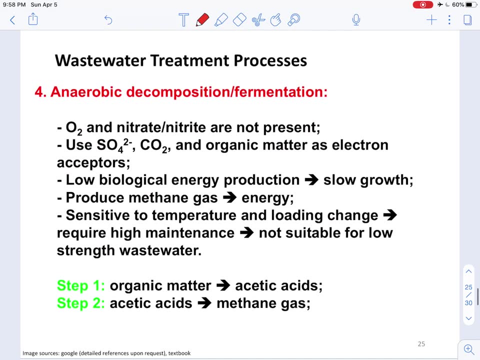 denitrification. so after we remove these nitrate or nitrite, basically they're converted into ammonia and then we can go back to the aerobic decomposition to oxidize the ammonia, to remove these nitrogen sources. okay, so the other decomposition type is the anaerobic decomposition or the 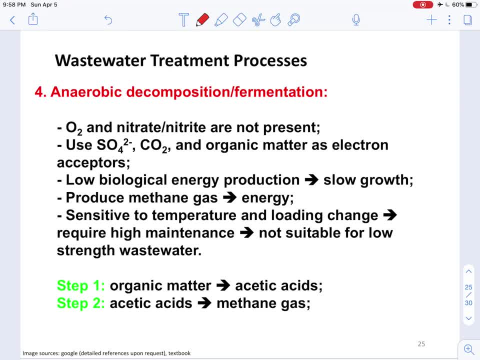 fermentation. so this is a process that does not require oxygen, or oxygen have to be absent so that the aerobic decomposition can take place. so the fermentation process will use sulfate ions, carbon dioxide or organic matter as the food right. so for this process. they are typically under low biological energy production, which means that it's going to produce less. 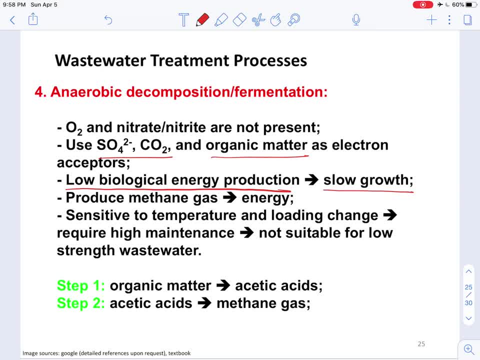 energy, so that's going to give a slower growth of these microorganisms and they also produce methane gas. so methane is kind of a lower level of energy there. okay, because if the, if the process is as fast as the aerobic process, they will further oxidize these methane into carbon dioxide and water. but here 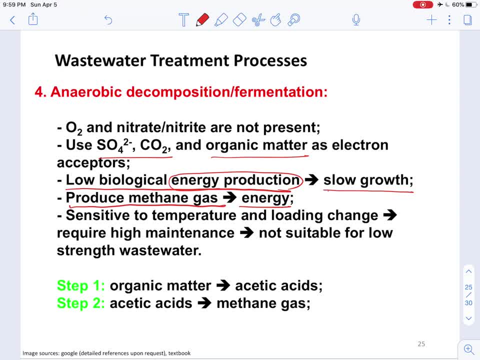 for the anaerobic process or the fermentation process, they're just going to give methane gas. there's no way they can further oxidize those. so and also for this anaerobic decomposition. they're sensitive to temperature and loading change. they require much more maintenance and not suitable for low 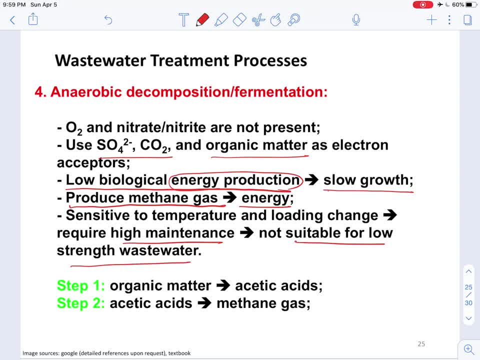 strength wastewater. okay, so they just so. if the water is very polluted, then it's better to use these anaerobic decomposition- okay, so there are two steps for the anaerobic decomposition. so the first step is to convert these organics into acetic acid, and then the acetic acid will further get converted. 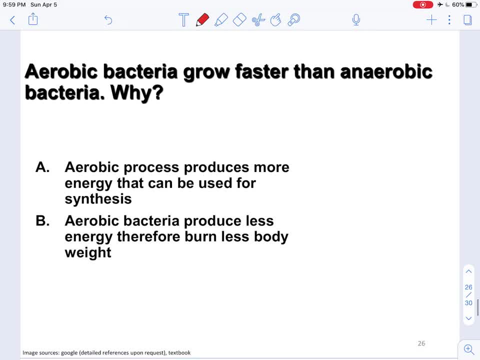 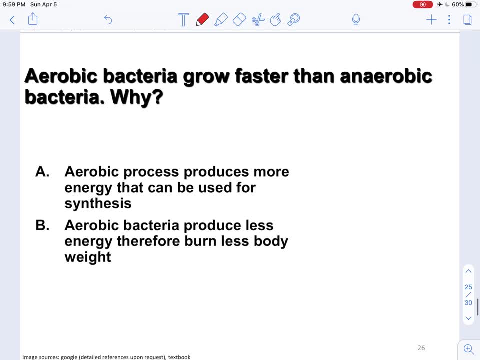 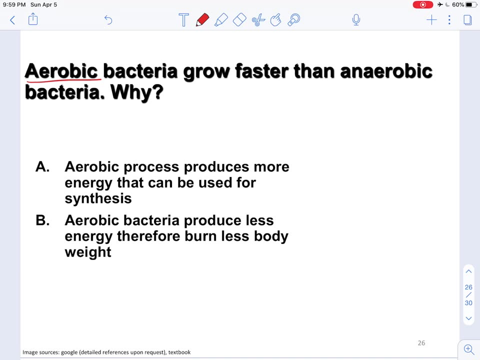 into methane gas. so here's a question. it's asking why the aerobic bacteria grow faster than the anaerobic bacteria, so we introduced that. the major difference between these two decomposition process is that the aerobic decomposition generates much more energy, which means that it can sustain more cell growth. right, so because of? 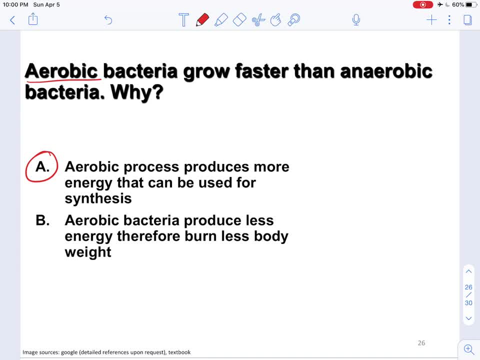 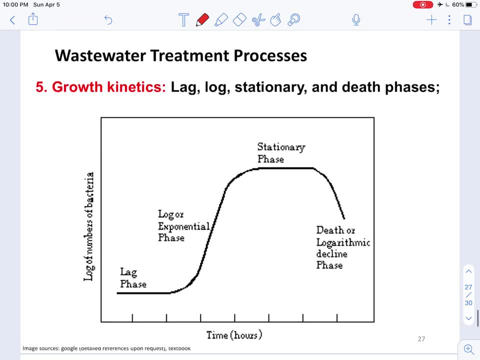 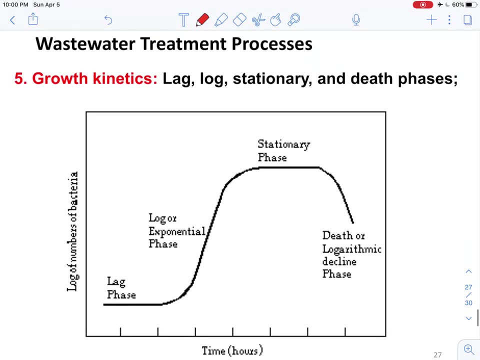 that we should choose a here. the aerobic process produce much more energy that can be used for synthesis. okay, so finally, we're going to start a little bit on the activated sludge. so we introduce that we can in. we can add these microorganisms in wastewater to let them help us. 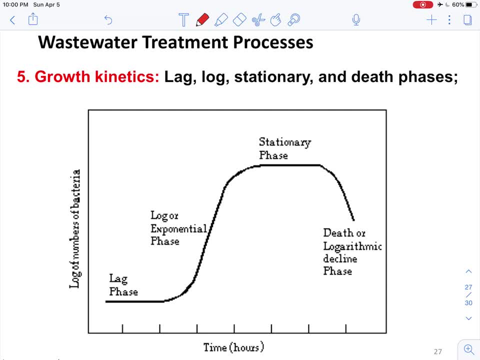 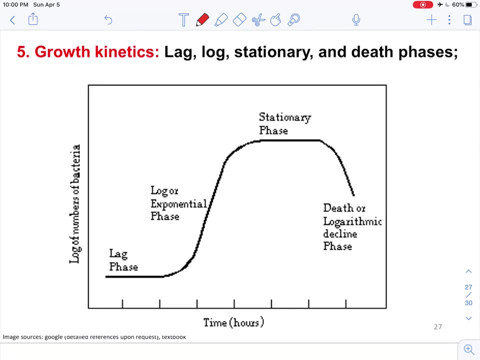 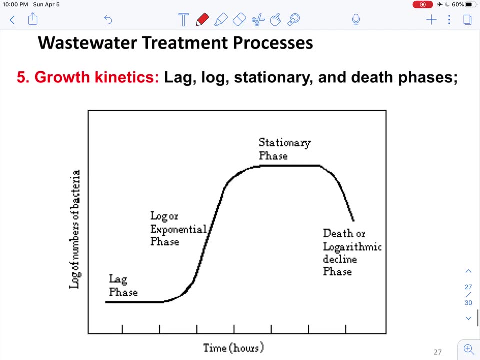 decompose the organics in the wastewater. okay, so because of that, we need to know what is the growth curve for these microorganisms. we introduced earlier in this semester that in terms of the growth or the population of these bacteria, or into these different phases, right, So we have lag phase, which is the initial phase. 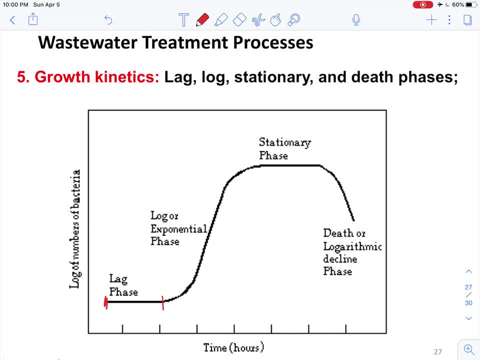 that the microorganisms are growing, but they're growing at a smaller speed. So we then have the log- normal or the log or exponential- phase, where the number of the bacteria increases significantly, And then we'll go into this stationary phase where the rate of the decay 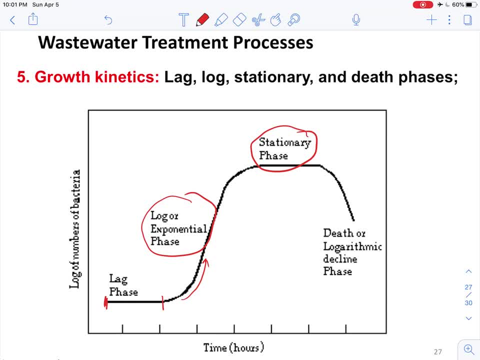 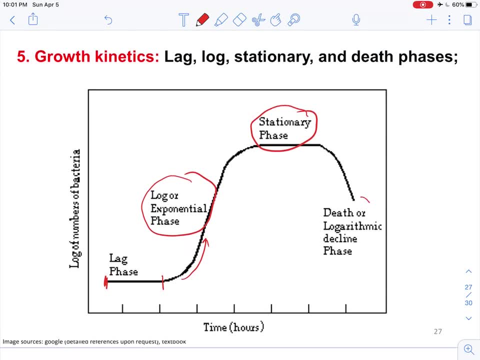 or the rate of the microorganism dying is equal to the rate of the new microorganisms being produced, And then if all of the food are being consumed, then they will go through this death or logarithmic decline phase. So actually this curve kind of reminds me. 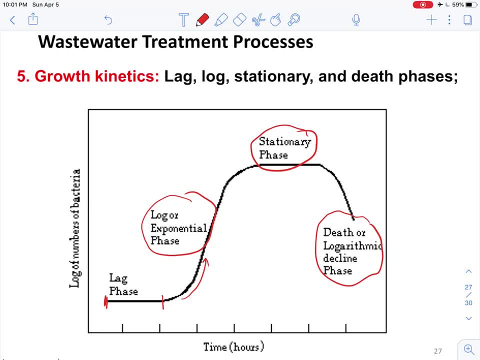 of these current COVID-19 situations here. So if you track the number of the people getting diet, getting this disease here, You can see that we're also seeing these types of curves. That's why people are mentioning that this slope going up is going to be much faster than the slope going. 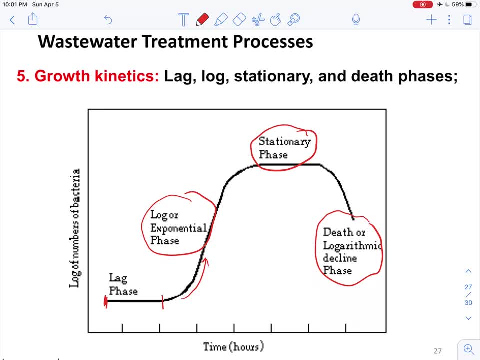 down. So that's what right now our country is trying to do. It's trying to really push this curve further. this way We call that flatten the curve So we can have a slower growth. So we're not saying that of course it would be great if we can reduce the total population that's getting. 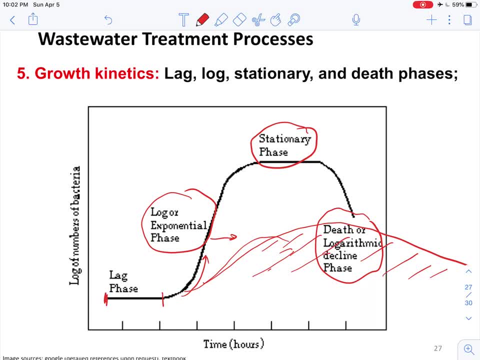 transmitted by this virus here. Actually, that is what we're trying to do. We're giving the stay-at-home orders, We're giving recommendations to put on masks, So we're really trying to reduce this number here, But also we're trying to push this curve. 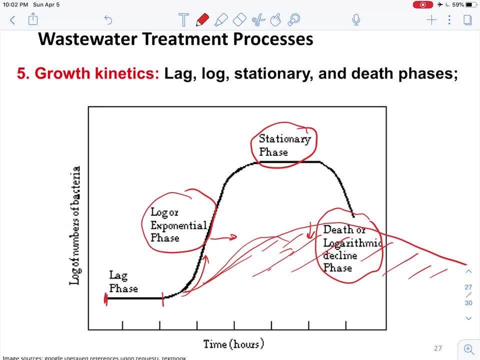 more flattened so that the hospitals have the resources to take these patients here. If all of the patients are going in this exponential curve, then the healthcare systems or healthcare facilities are going to explode. There's no way they can handle this large amount of patients here. 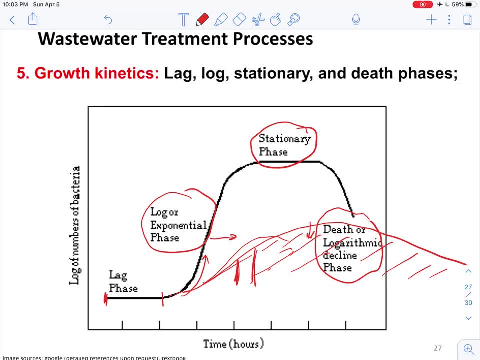 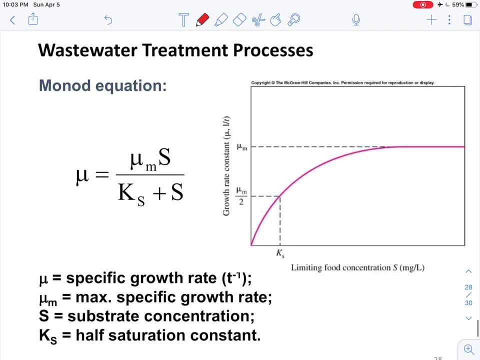 So, although they might be having different types of growth kinetics- because I'm not an epidemiologist, but by looking at this curve here it really reminds me of what is happening right now in our country In terms of how to predict the kinetics here. 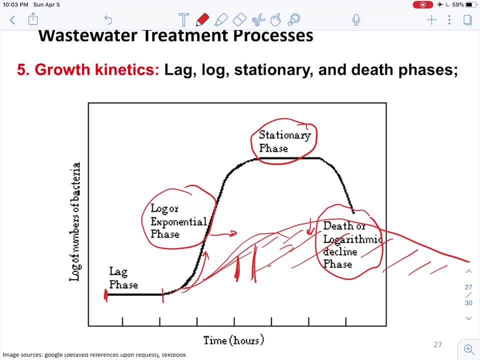 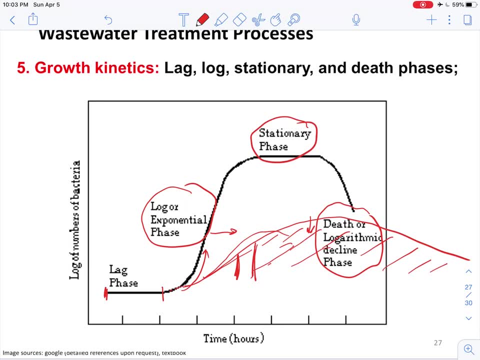 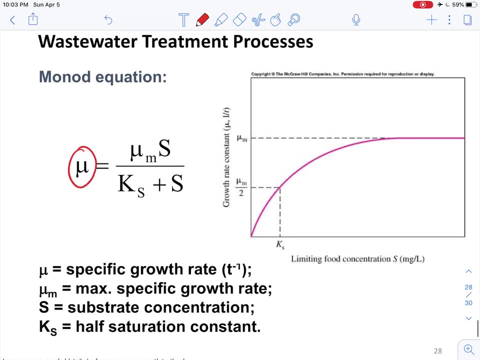 the growth rate here. So right now this is just showing the number of the bacteria. So if we know that, if we take the derivative of this curve here, then we're going to obtain a growth curve, obtain a growth rate. so basically we call this growth rate as mu here. okay, so 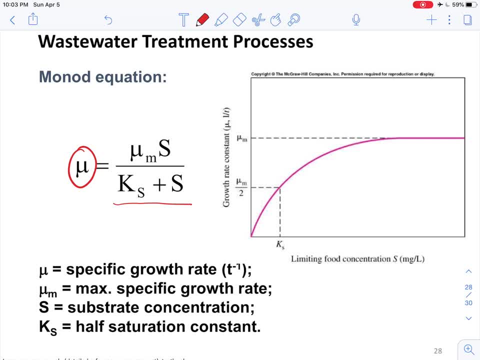 the mu can be calculated by different parameters in showing this equation. so this equation is called the Monod equation. so what the Monod equation means is that the growth rate of the bacteria really depends on how much food there are. so let's imagine there if there's an unlimited amount of food in. 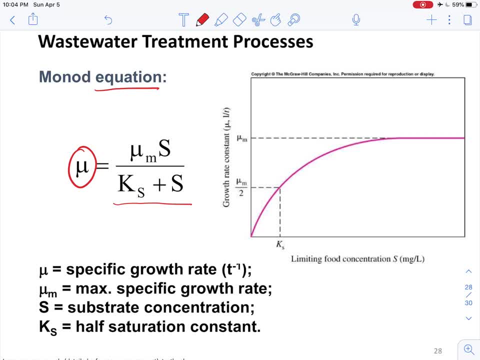 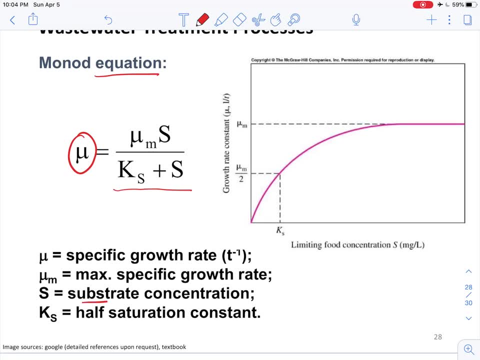 the system, then the bacteria can grow happily, right, they can grow at the maximum speed in terms of their population. so in this equation, S here represents the substrate concentration, which is the, the organics in the water. so that's the food of these microorganisms, right? so you can see that. 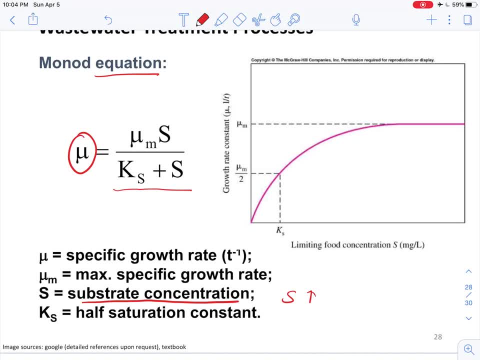 if the S goes to infinity, what's going to happen in this equation? so if the S go to infinity, they are going to be much larger than the KS. so these thing can two S can cancel out. we can obtain this mu M here. so mu M is a maximum specific. 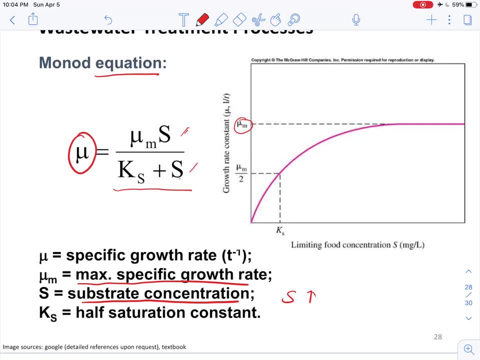 growth rate. okay, but typically there will be limited amount of food, right, so that's why we were seeing this reduced growth rate. okay, so we further introduce this KS here, which is a half saturation constant to describe this curve that's happening here. okay, so you can see that if the S is too small, if the S goes to, 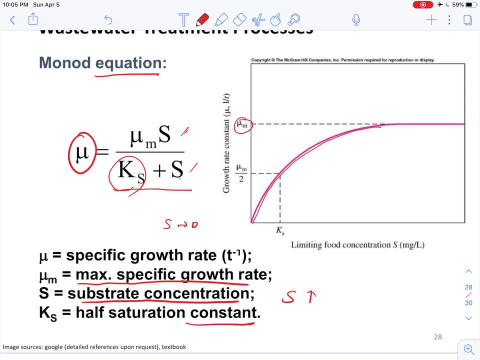 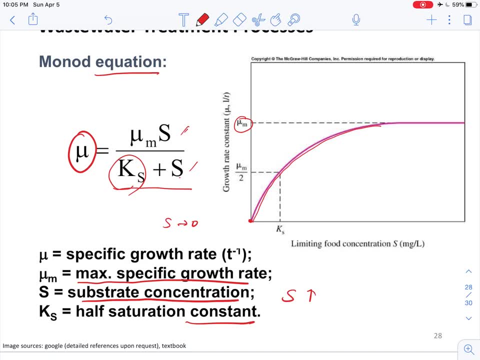 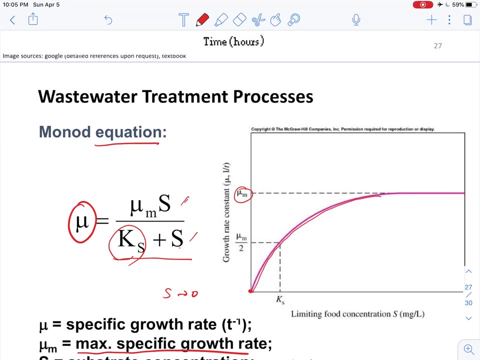 zero. what's going to happen? the S goes to zero, the denominator is KS, denominator is zero. so basically, the growth rate will go to zero. okay, that's, it's the point here. all right, so the model equation really, really describes what is the growth rate of the bacteria, the growth rate of the 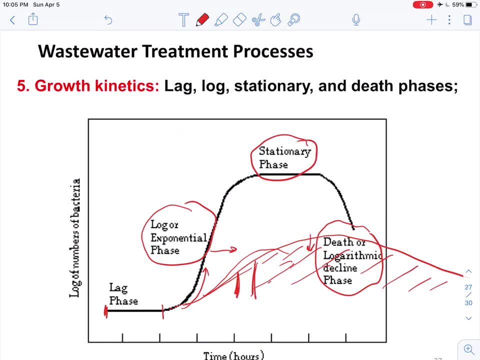 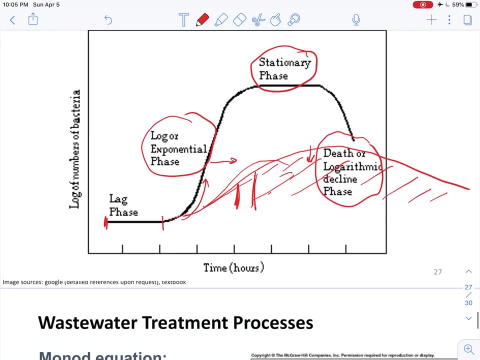 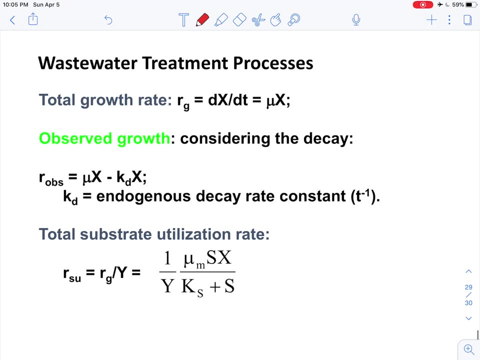 population of the bacteria. but if we look at the population here, it's not only the growth that's driving the population. there's also decay or the deaths, or the death of these bacteria. okay, so if we just consider the growth of this population here, then we can tell that the growth rate RG is. 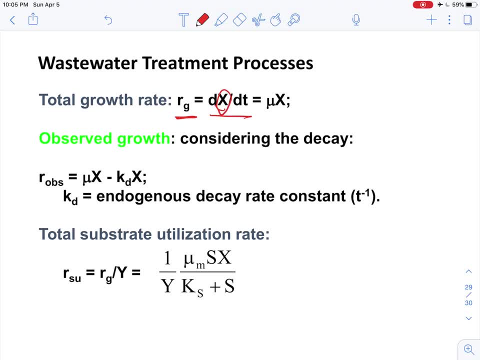 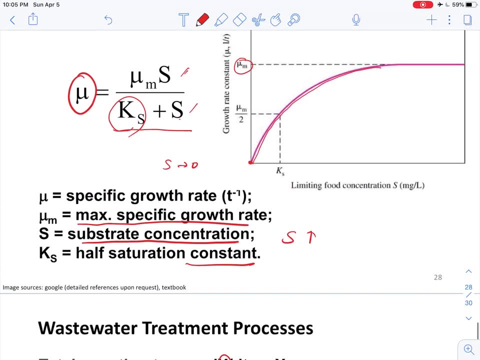 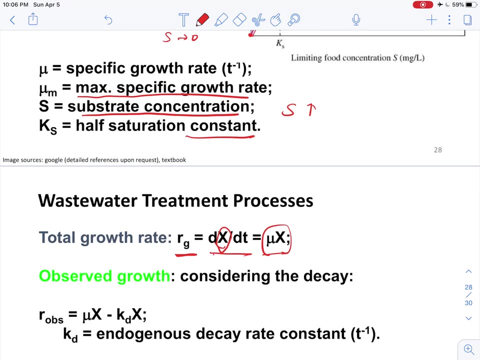 equal to DX divided by DT, where the X is the population of the bacteria. okay, so that is calculated by mu multiplied by the X, and this is a first-order reaction. okay, so this is a first-order reaction. okay, so basically, the population or the change of the population for the bacteria is: 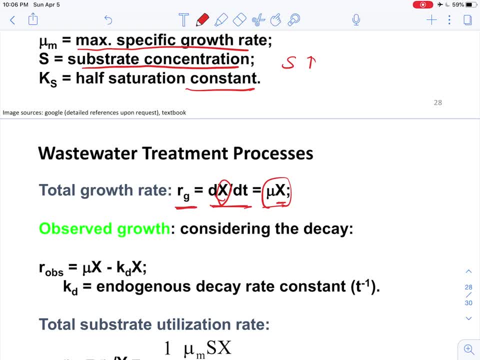 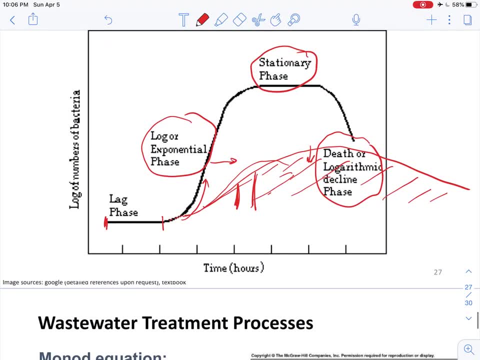 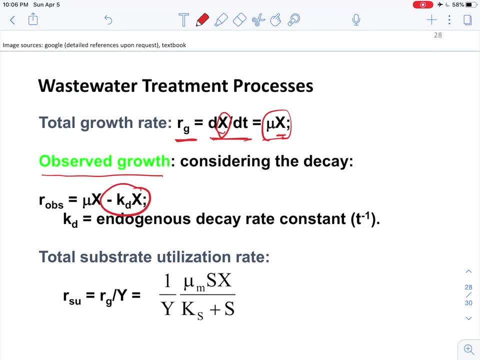 equal to the growth rate multiplied by the concentration of the bacteria. okay, so there's also a observed growth. so the observed growth is what's happening really in this curve here. so the observed curve, observed growth, have to incorporate the death or the decay of these microorganisms. we call these as. 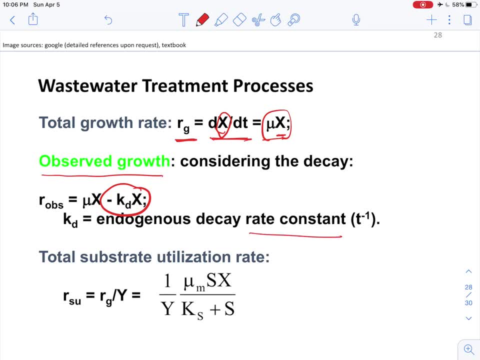 endogenous decay decay rate RG to one second. so we have to make sure we have rate constant. So because of that then we can tell that dx dt is going to be equal to this term here. So people also design or define a parameter called the total substrate utilization. 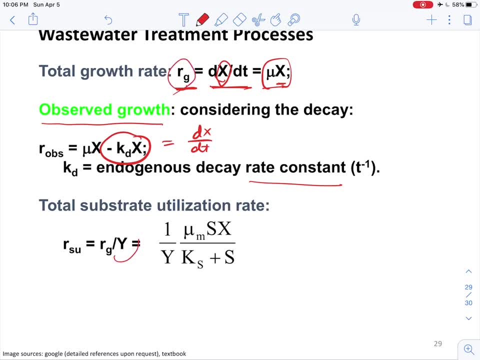 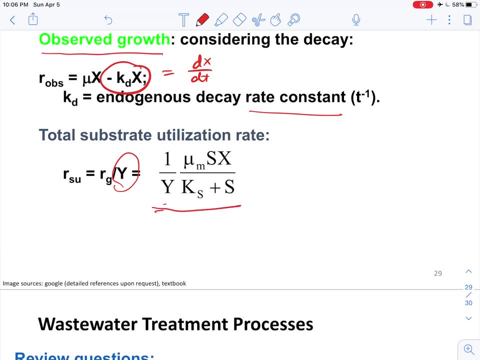 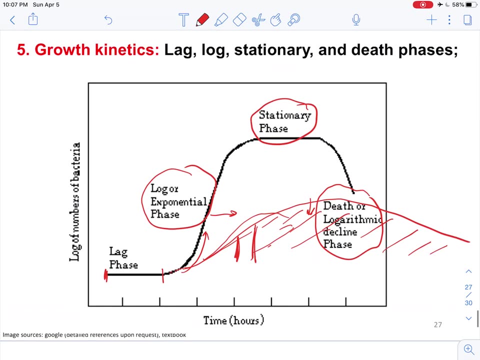 rate. So that is dividing this growth rate by the substrate concentration or the amount of food. So that is going to create us a new parameter here. So we're going to show how we're going to use these parameters to describe the population of these bacteria or microorganisms and also how 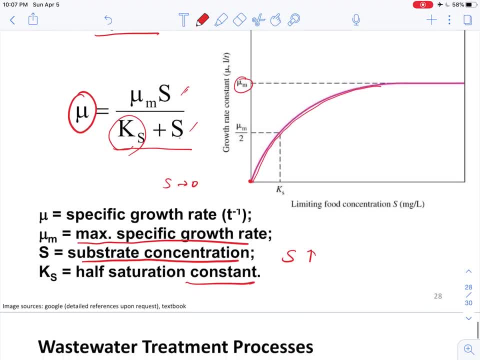 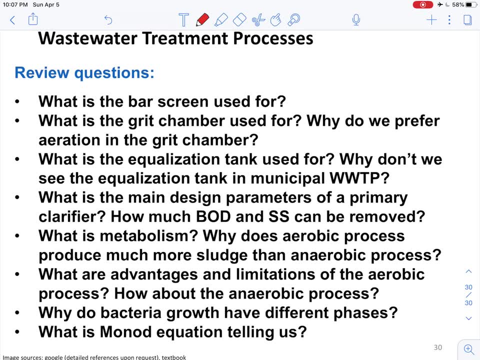 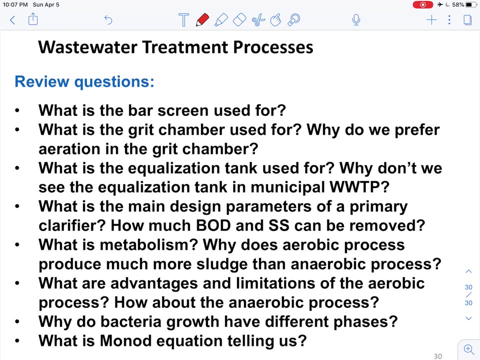 we can design the activated sludge process to treat the wastewater quality. So that's all for the contents of this class. So, just as a review, so we need to understand what is the bar screen used for? what is the grid chamber? what is the mechanism? 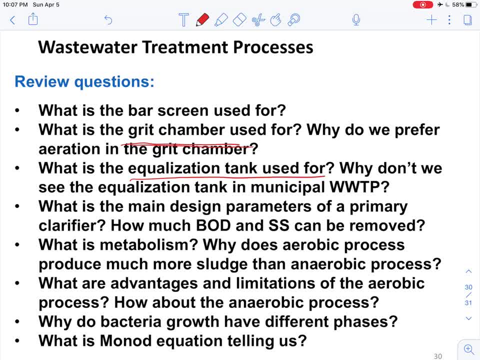 of the grid chamber right, What is the equalization tank right? And also, what are the main design parameters for a primary clarifier? What is the metabolism? What are the advantages and limitations of the aerobic process? Aerobic process is the process that needs oxygen, but we cannot use that. 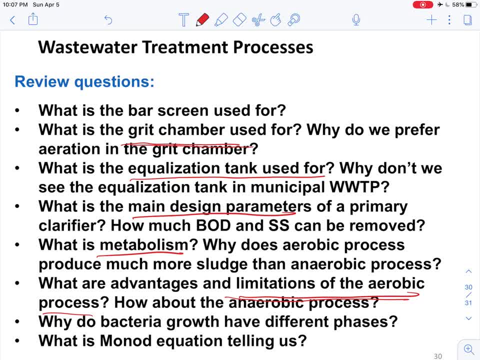 for wastewater that has too much organics inside, because that's going to require too much oxygen. so we need to understand how the bacteria grows, have different phases, and also what is the model equation. What does that tell us? Okay, so that's all for the contents of this class. Feel free to 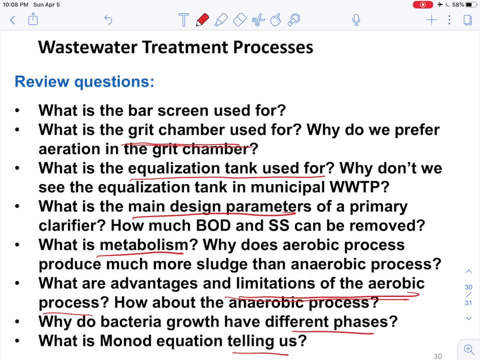 let me know if you have any questions and talk to you on Wednesday. Bye.